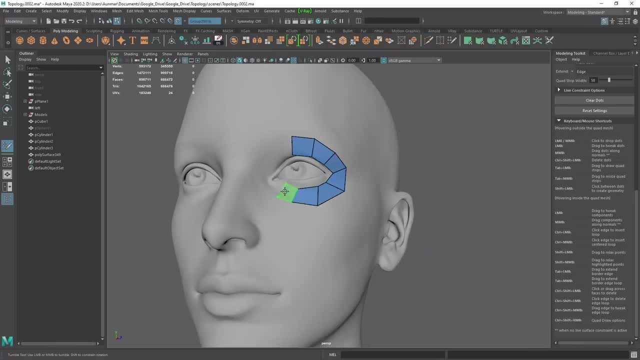 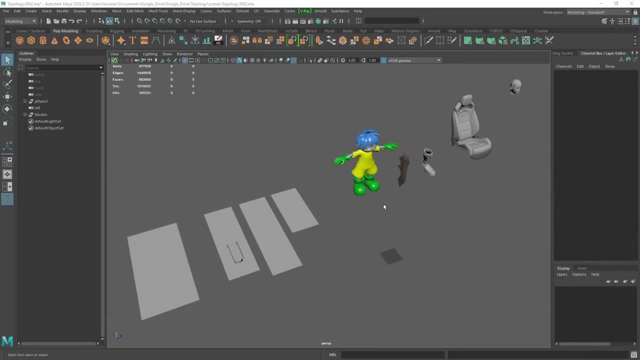 As always, a like and subscribe is always appreciated as I continue to grow the content of this channel. So with that, let's get started. Alright, so here we are in Maya, and I'm going to start with the very first tip And the first. 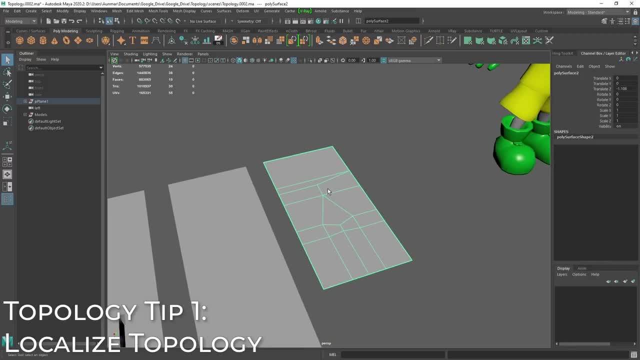 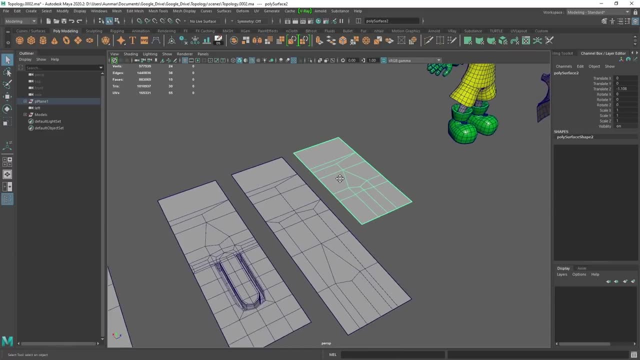 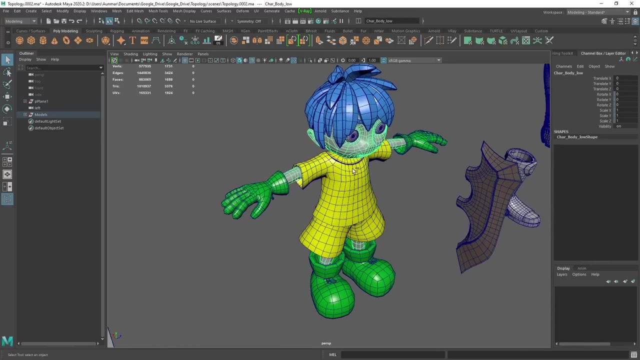 tip is localizing topology, And what I mean by localizing topology is having the ability to add topology within your model without spreading topology and edge flow in areas that you don't want. For example, if I go ahead and take a look at this hammerboard that I modeled, 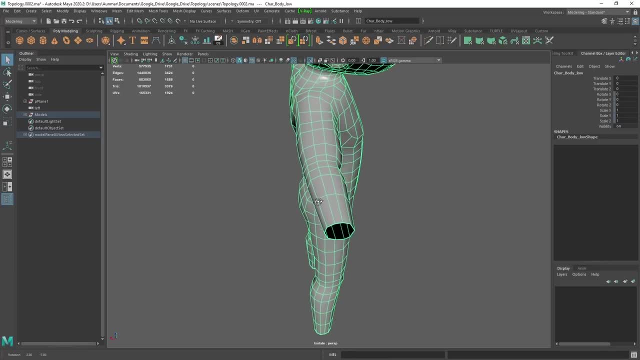 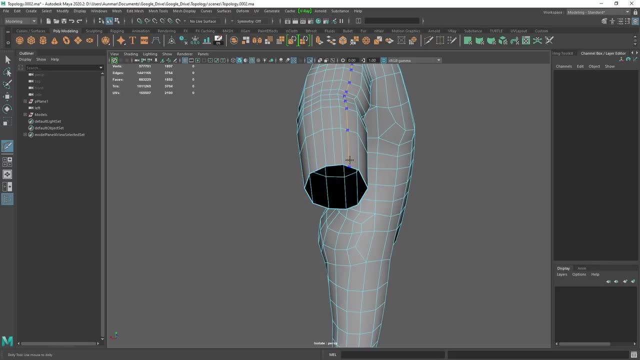 before. I can see that the topology in this model is a little bit different In a previous tutorial and I want to add geometry here for the hands. The last thing that I'd want to do is to jump over to multicut And just to just add in edge loops here that are 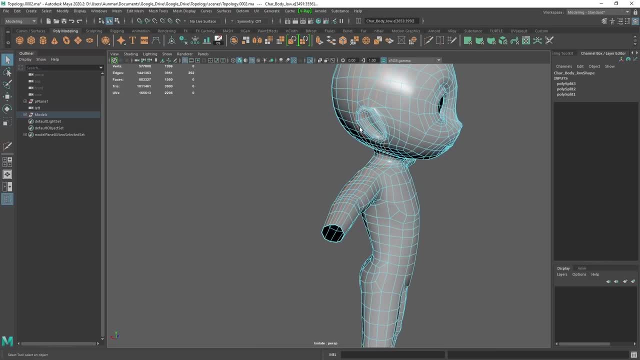 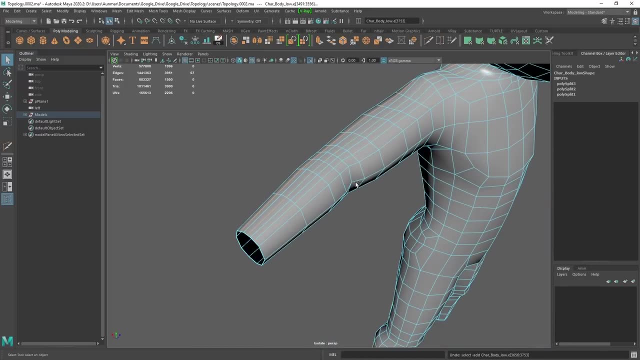 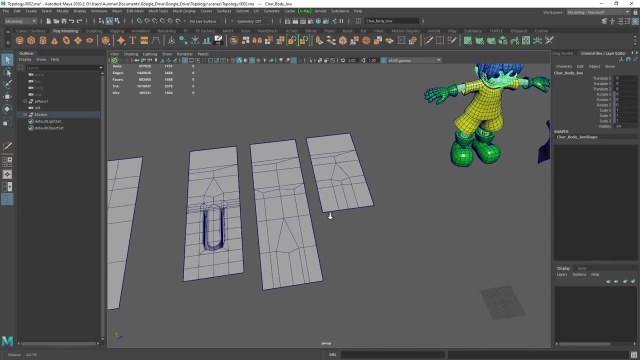 now going to run the length of the model, right, And you can see how this gives me unintended edges that run all the way around the model. I definitely don't want that. So what I want to do is me undo that, jump back to this plane here And I can show you kind of a simpler, a simpler. 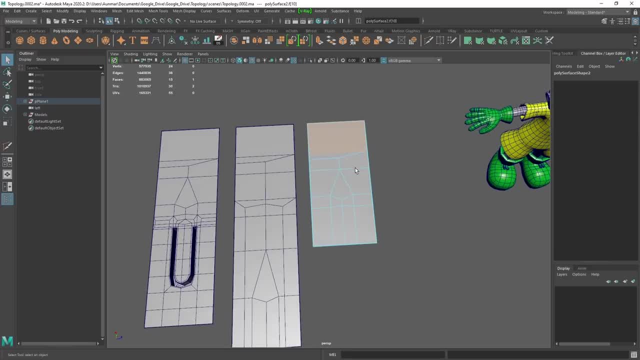 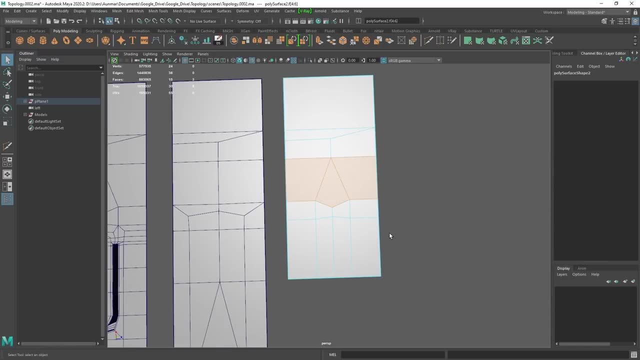 point of view. you can see that I have one face here that's being cut and split into two faces, And then it's then being split into even more faces here, So now we have 1234.. So we started with one And now we have four. you can see that I can combine that with different techniques here. 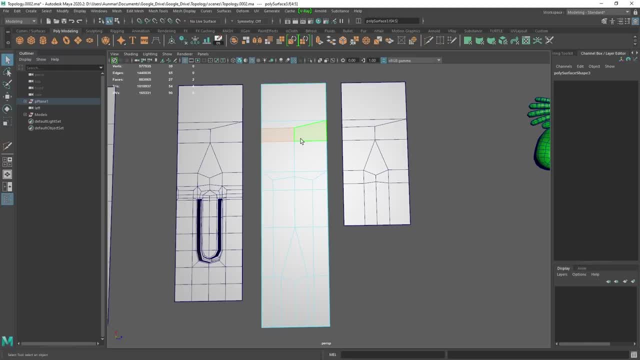 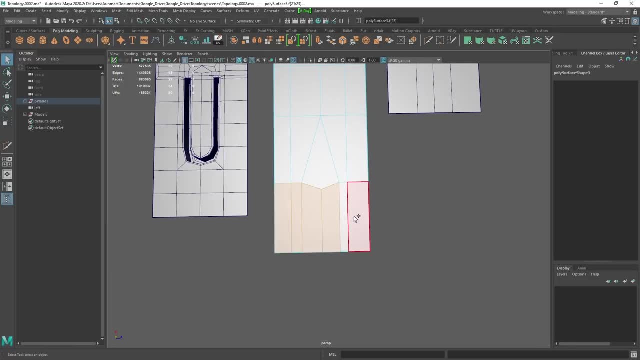 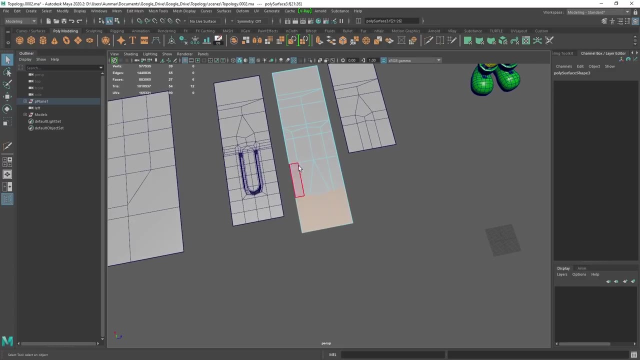 where I start with one face, end up with two and then split that to have four here, And then now I can even get almost six faces here, Right, And so this is just allowing me to add topology strategically right, and localizing it in areas that ice only need it. Now how would I do? 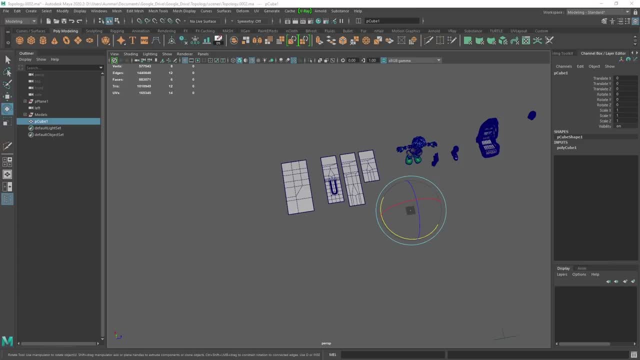 this: if I go ahead and create a cube here, we can go ahead and take a look. I'll go ahead and scale this cube up And zoom in And we'll go ahead and just do a Ctrl E for extrude and then do an. 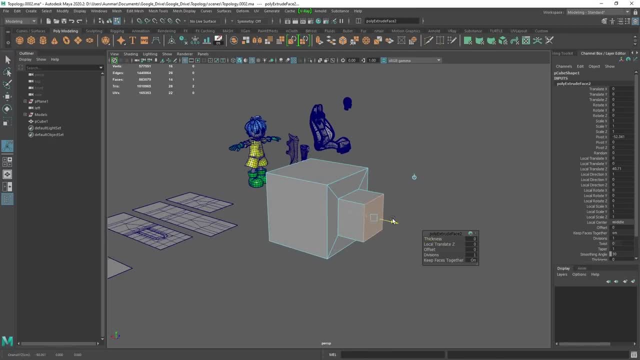 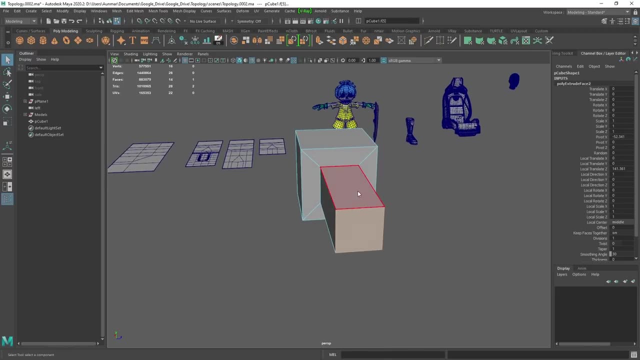 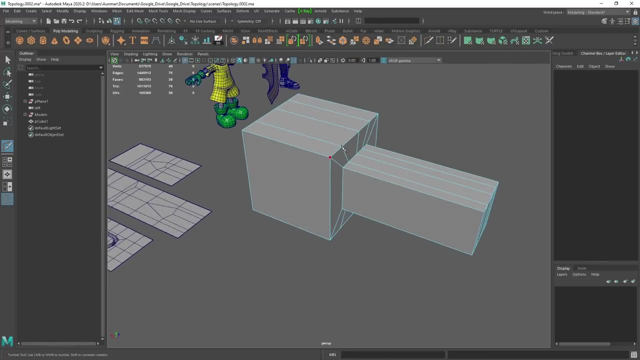 offset, bring this in and then hit G to repeat last and then extrude that out Now again. if I wanted to now extrude some fingers on here and I go ahead and do the multi cut, we can see what happens if I just start adding in a bunch of edges that are now routing throughout the rest of 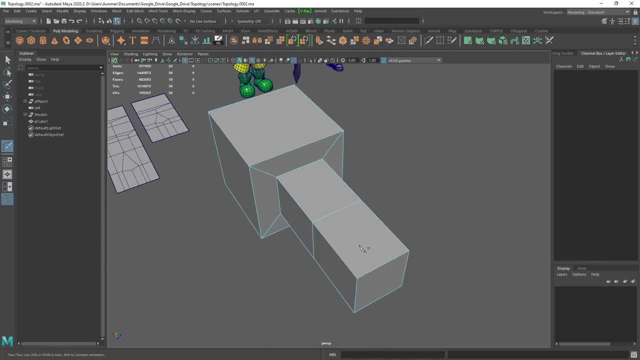 the model. So instead what I can do is I'll Ctrl middle click, add that in the middle and Ctrl middle click again, Now one thing that you can do. there's a couple ways of doing this. you can add Ctrl middle click a few times here, like so, Or I'll just go ahead and left click a couple of. 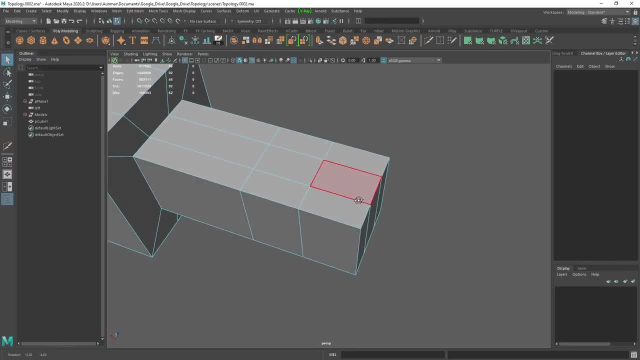 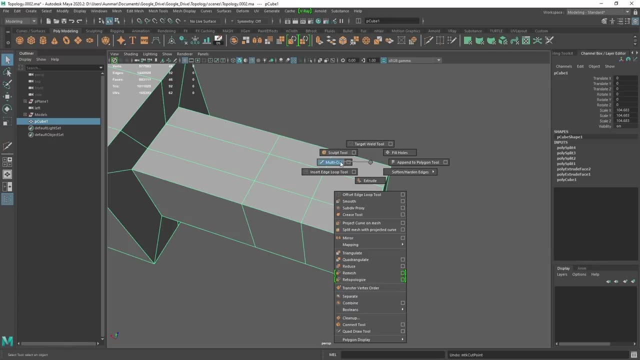 times. Now what we can do here is I can go ahead now and move these faces, And I can do that by entering the multi cut tool. So if I grab the multi cut tool, I can start at one corner and cut about in the middle and then start at the other corner and cut at the middle here, Like so Then? 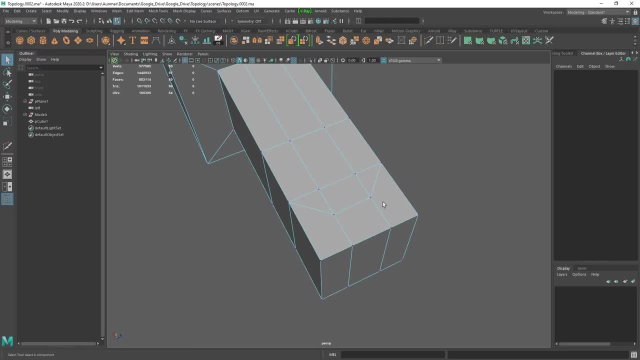 I have this Now, of course I'd want to just kind of meet these or connect these two. Then I want to remove these edges here, like so: Now we have these or this face loop running around And that allows me. 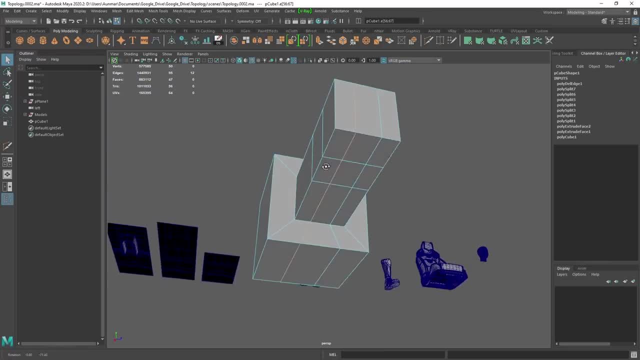 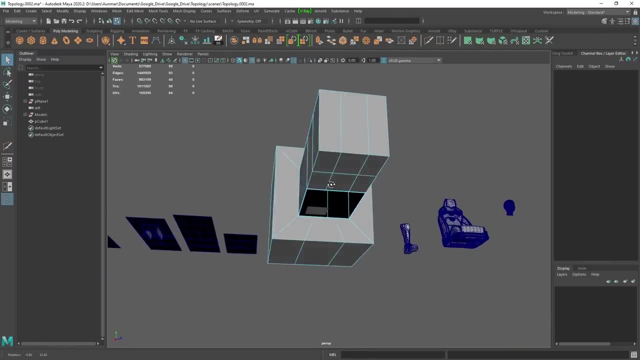 to be able to go through and delete these edges. Now I want to make sure to do the same thing on the bottom, But for right now, I'm simply just going to delete these faces, So it doesn't loop all the way around, for the simplicity of this demonstration. So I'll go ahead and select these. 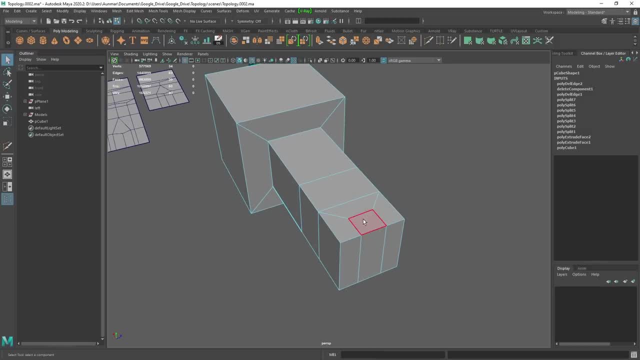 edges and then right click on them, And then I'll go ahead and select these edges and then remove, And then now you can see that I have these faces here here without adding all that extra geometry in on the rest of the mesh, And you can combine that with techniques again, if I go. 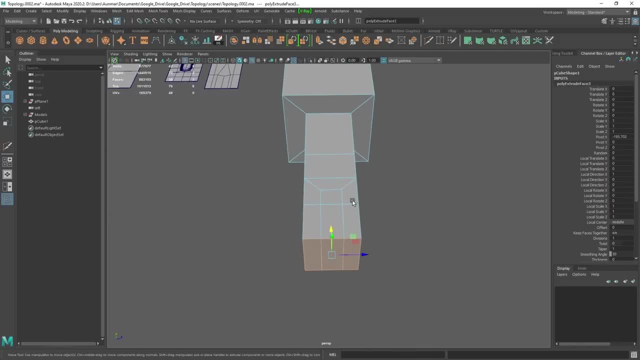 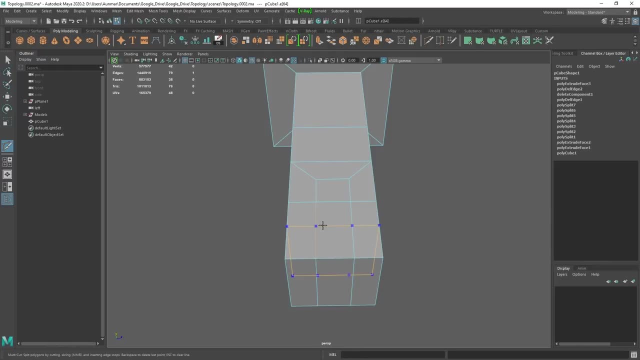 ahead and just kind of shift, move this to extrude. And if you wanted to even add even more, you could grab your multi cut tool again And I can middle mouse cut that. And then you can do something like this: where we call these- I call these kind of kites or diamonds, like so- And now I can go ahead. 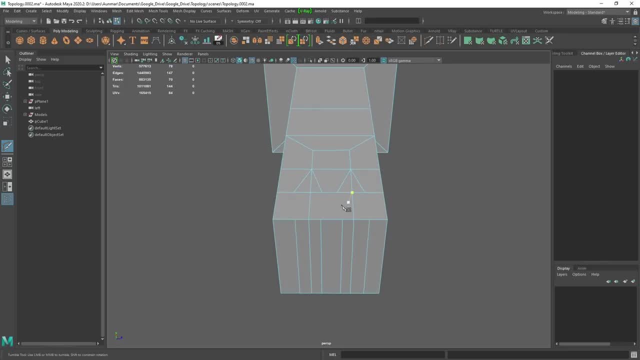 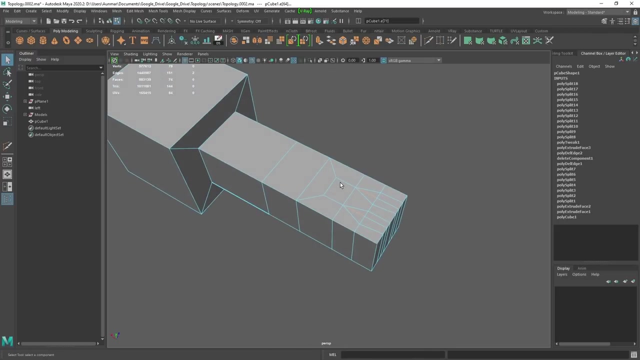 and start to add in more geometry or edges here. right, so, like so. Now, what this is going to do is allow me to have a bunch of edges or a bunch of faces here, without again taking it throughout the rest of the mesh, And then now, even though you can see that I have, 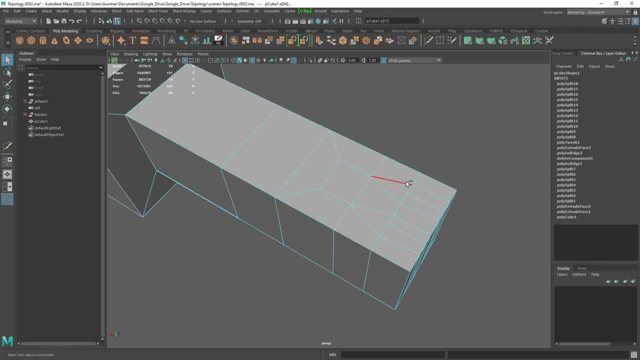 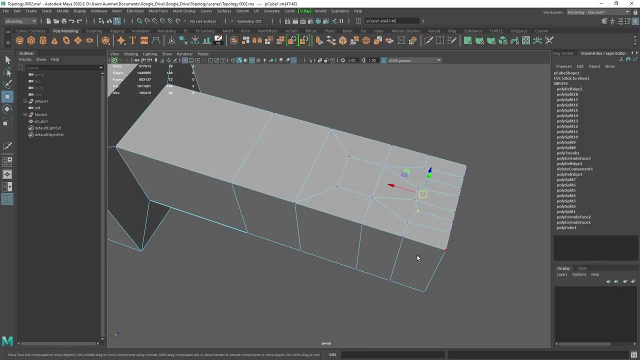 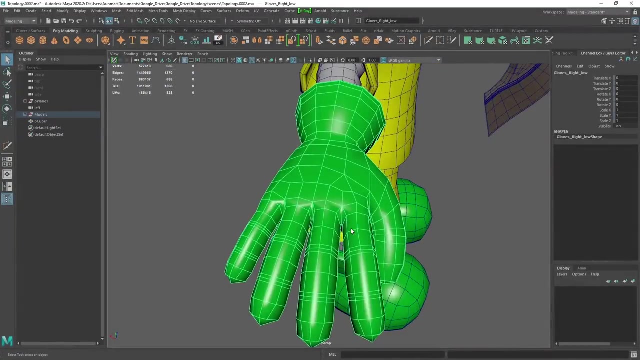 these triangles here. I can simply remove this middle triangle here and create the kite kite shape that I was talking about, And then now I go ahead and just kind of move that and then there we go, And again you'll see this being used all over the place. I use these all the time for. 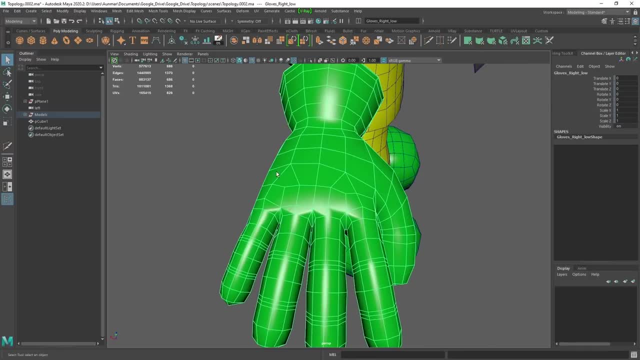 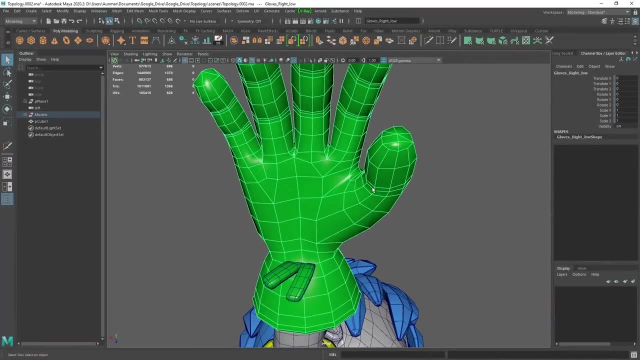 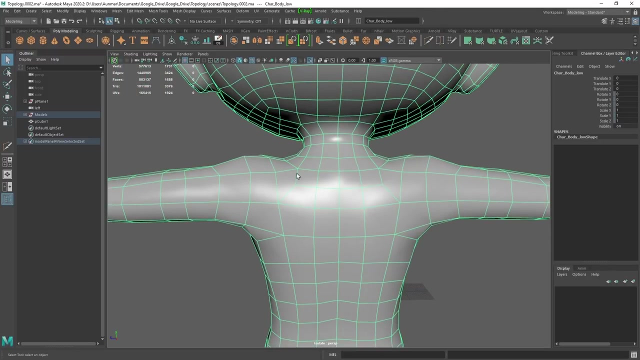 hands, So you can see that I have this kite shape here. That's just allowing me to add in some extra geometry for the fingers without having to go through and add it throughout the rest of the glove or the rest of the model. You'll see me use that here as well, on the back of the model where I start to use this. 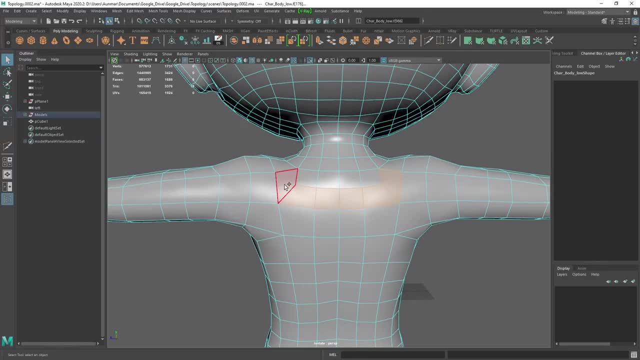 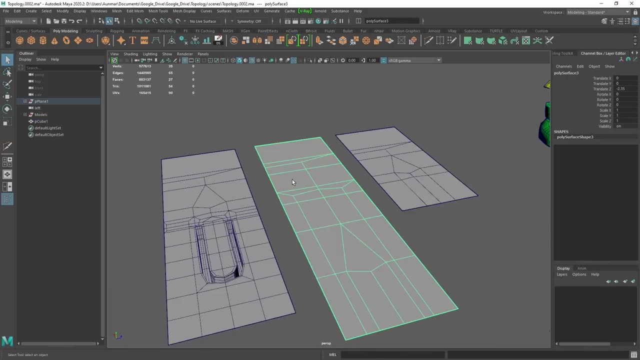 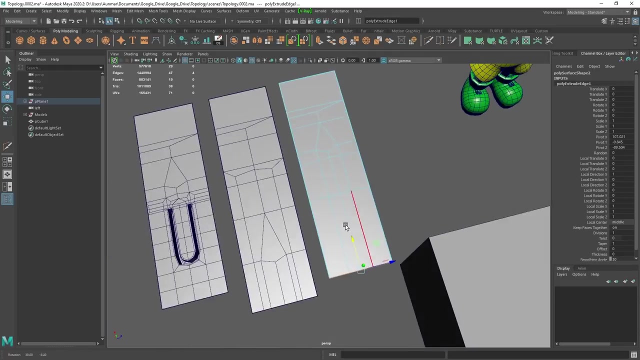 inner part, this face loop, to be able to add in some more geometry. And again, kind of the last thing here is, if I go here now, you know you can go ahead and move this edge, like so And you can kind of just manually do it. where you're a multi, cut this. 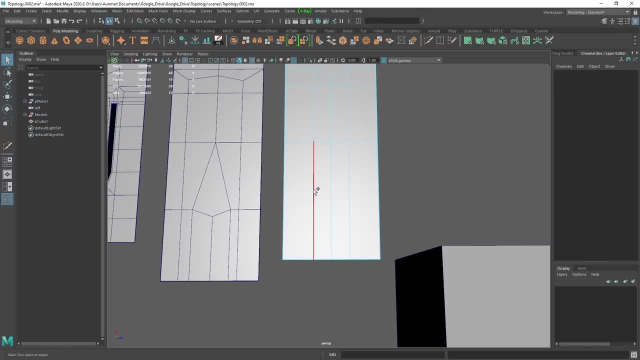 and go ahead and multi cut and kind of add in a point here. That real quick And you can just manually cut in to get these loops too. So that's another way of kind of doing the same thing. So I do this all the time like so, and then I can terminate it at this edge. 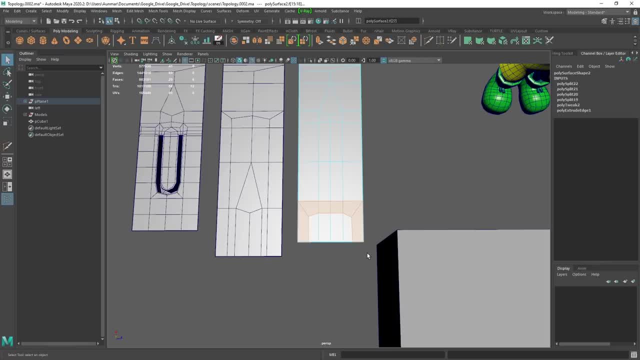 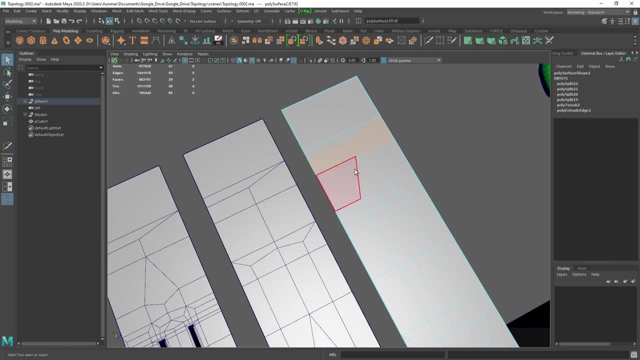 And again you get this nice face loop running all the way around. So, being able to understand the shape of the face loop and then be able to get the shape of the body and then do the same thing here And again, I'm going to show you how I go over this and how I do this, How to kind of start. 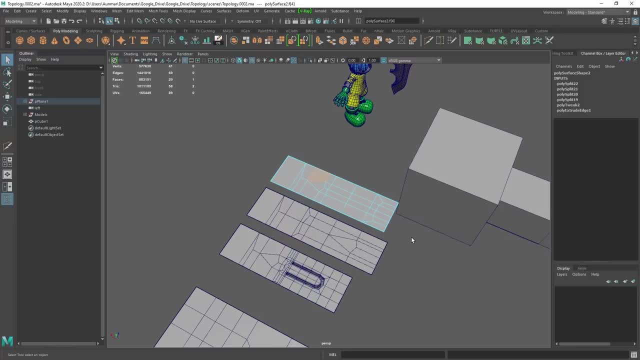 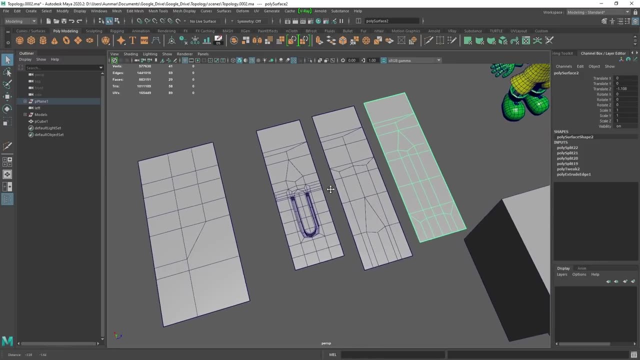 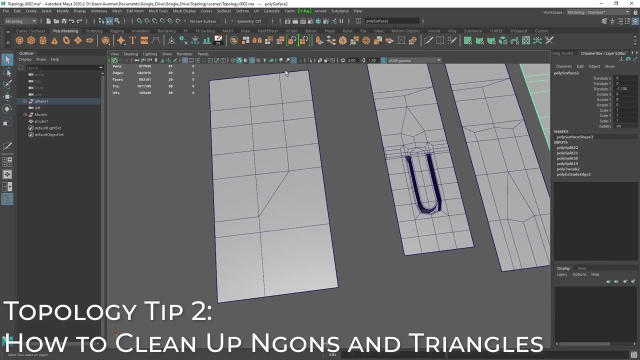 with one and split your edges and get more, or split your faces and get more edges to add that topology. This is what I mean by localizing topology. So using this technique is something that I use all the time. using these kite quads is something that I use all over my models. So the next tip is how to clean up end guns and triangles. A lot of times you'll be splitting and cutting faces and cutting some edges and then and then just cutting the edges, And this is a good way to do that. 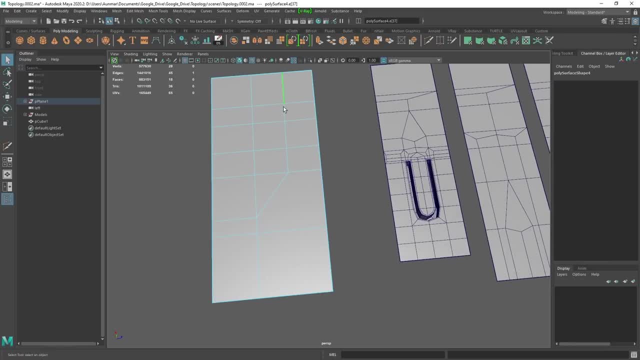 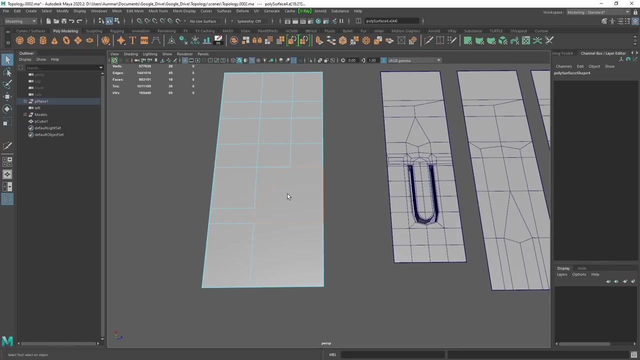 and cutting some edges and you'll get to a point where you're kind of running along and you have to diagonally cut across and then you're left with a triangle and an n-gon. So I get an n-gon, which is a five-sided face. Now we want to make sure at least for organic modeling and most of hard. 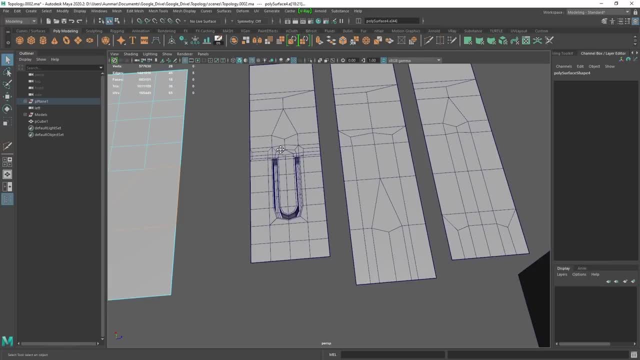 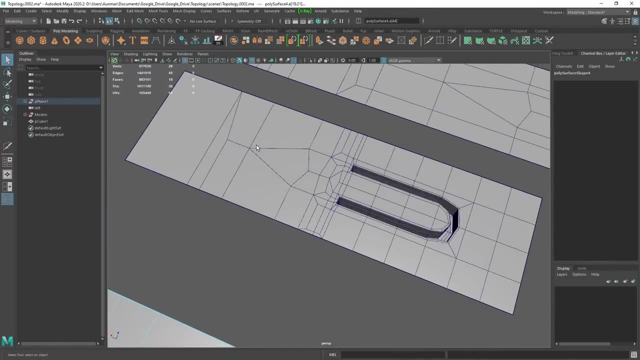 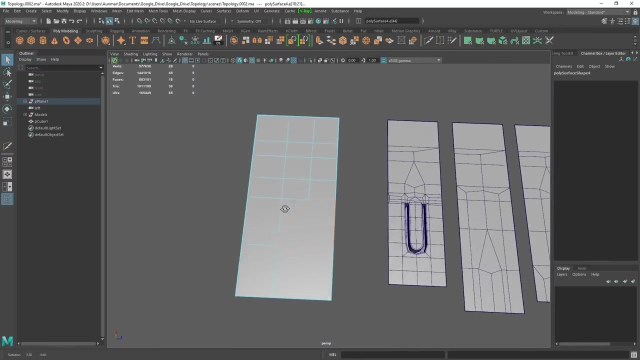 surface modeling, we want to typically end up with what's called just quads or four-sided polygons. You see that I have this, which is pretty complex, but all of these complex cuts and edges here are quads and they're four-sided. So when we get to this instance, when we're cutting across, 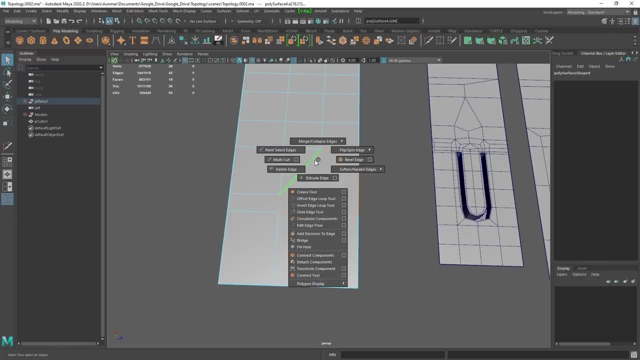 edges and faces. we can simply use this technique where we split this in half, and what I mean by that is, if I go ahead and jump into the multi-cut tool, I can just click on the middle part of the edge here and take it and terminate it at the corner. 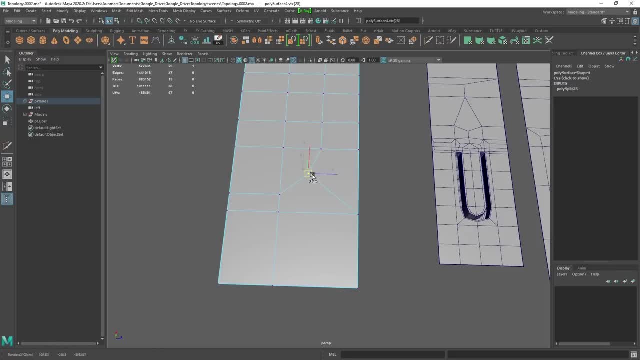 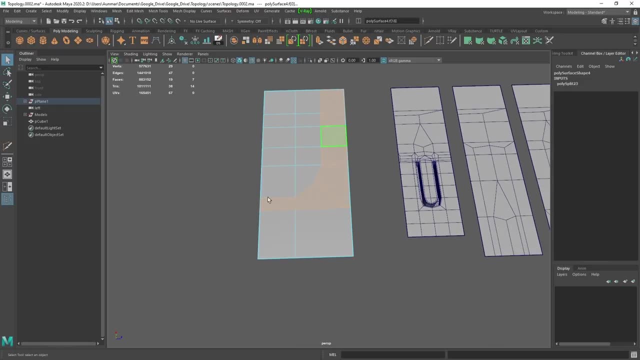 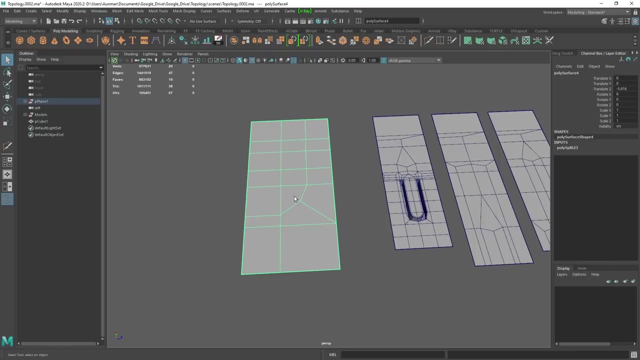 of that face, which gives me now this: I know this might seem very simple, but I'm telling you when you're going through and modeling and cutting and splitting. now you've just created this nice clean face loop that's running all over the model, which is exactly what you want, and it avoids a 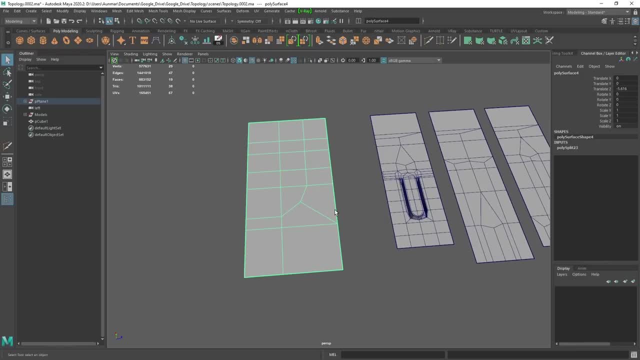 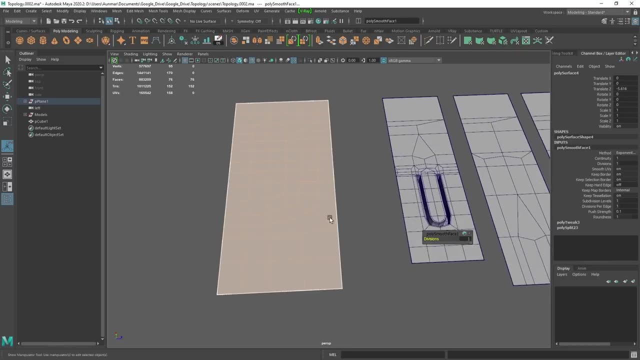 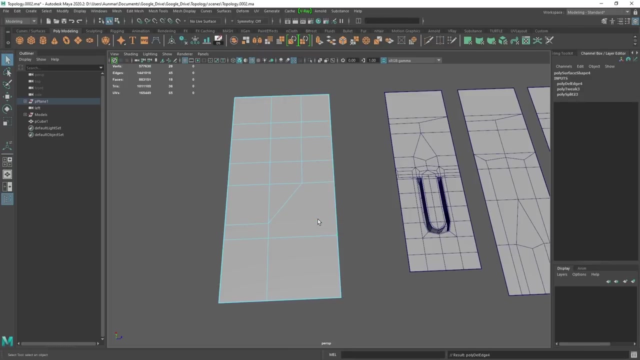 triangle and an n-gon, which both of those combine is going to give a lot of smoothing artifacts. So by smoothing I mean by holding shift, right click and going to mesh, smooth or smooth, and so you can see, you get these Nice, even quads, without that before. if I go ahead and actually just delete this, 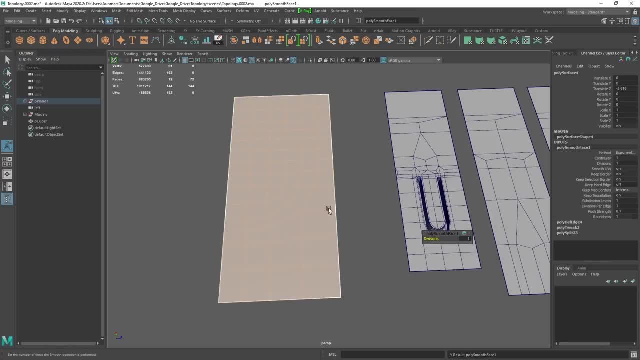 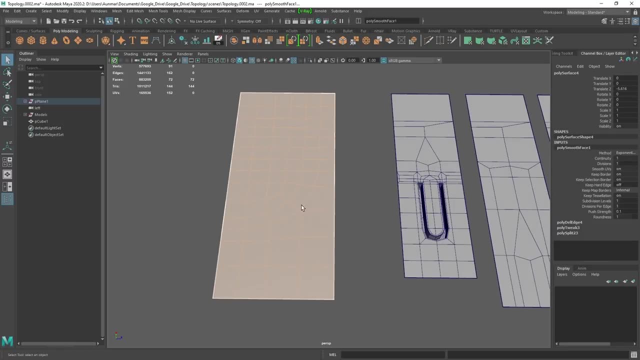 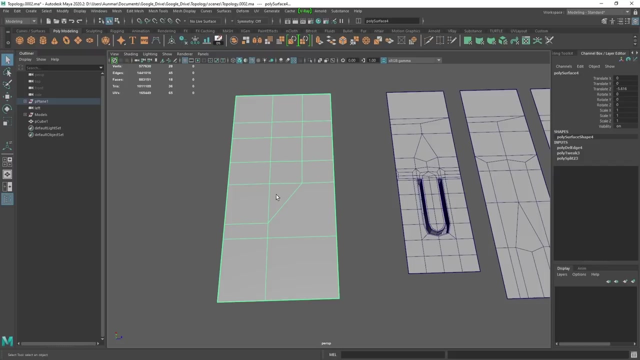 and go to the object mode and go ahead and smooth. you'll see it's going to try to do its best here, but it's giving us a little bit more uneven of a subdivision Now. so it's always going to subdivide, its best to try to end up with quads. but if the subdivision algorithm has to account for a lot of 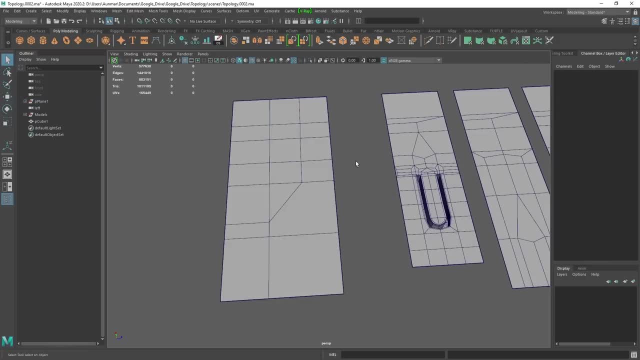 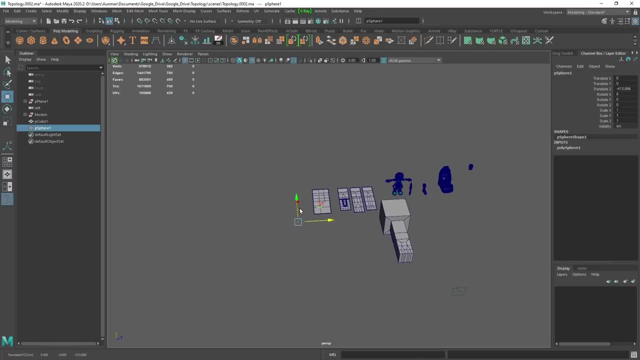 triangles and n-gons. that's what's going to give you artifacts, All right. so, for example, if I go ahead and pull open or pull up here this sphere and I bring this over and I'm going to scale it up, and I can go ahead and, you know, give myself a little bit more subdivisions, maybe something like: 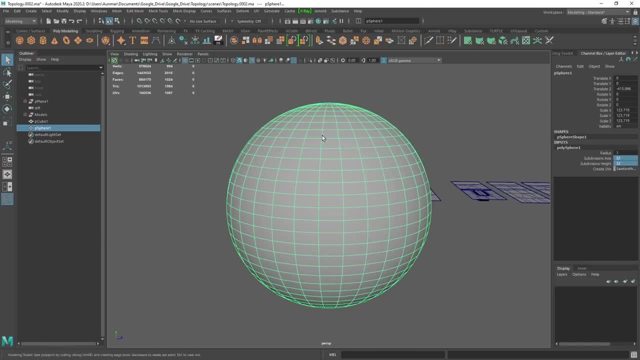 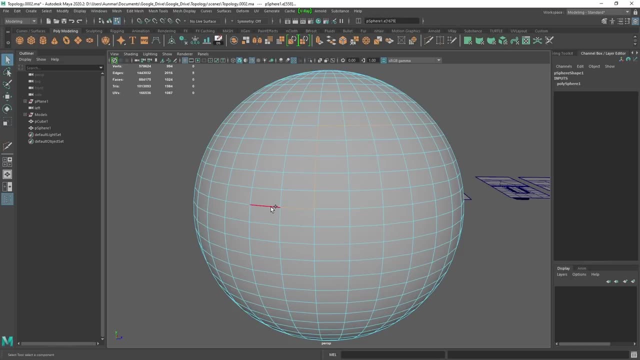 32, and this is you know where you can apply this technique. If I go ahead and start multi-cutting now, instead of just grabbing edges like this that are already on existing edges and working with that. well, if I wanted to do something more organic, I certainly can, so I'll go ahead and grab my 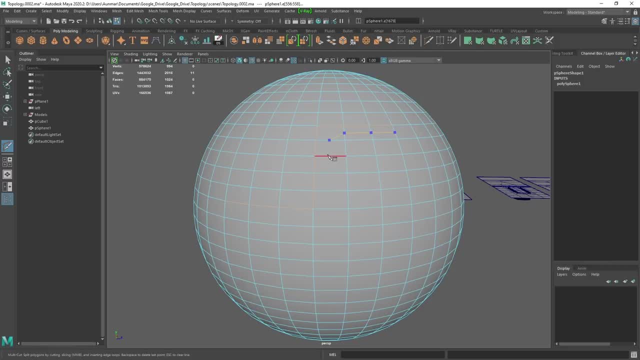 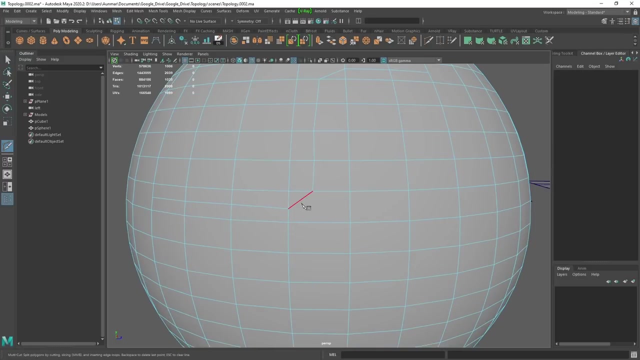 multi-cut tool. Just start cutting, and then now I can start cutting across edges, like so, and you get something like this: Now, again, you're going to be left with these triangles and n-gons, like so. So in order to easily fix that, we can go ahead and just split this in half, and split this top one in half, like so. 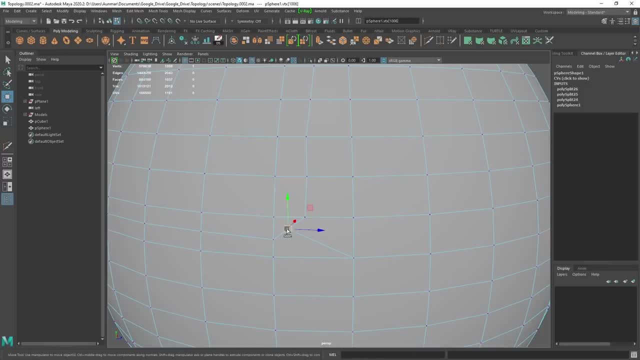 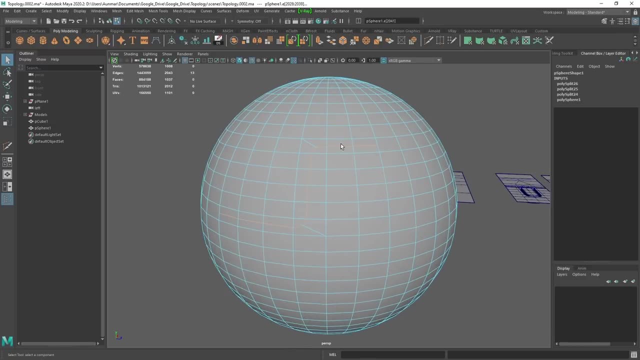 and there you go. We can kind of control, shift, slide on the edge, and then what we can get is selecting this edge. Now, obviously I'm not going to worry about where this ends up, but this is fine. and then I can hold shift, right, click and do a bevel edge. so you get something like this: 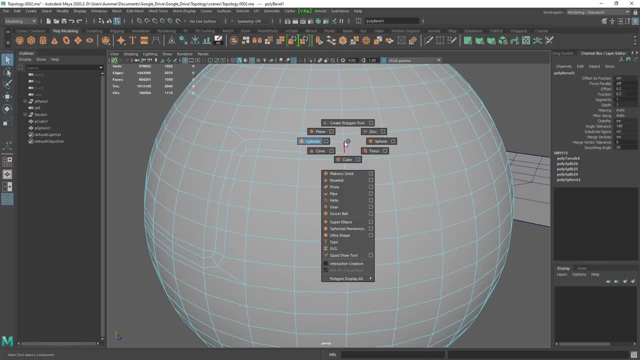 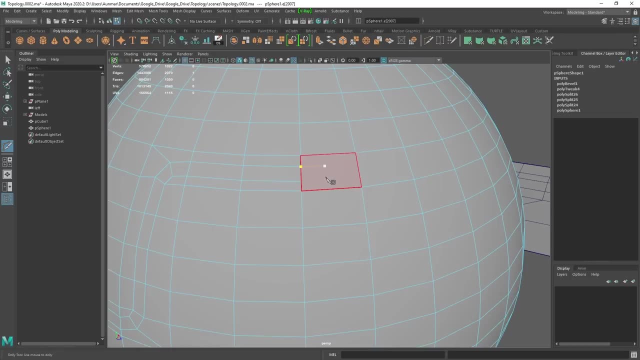 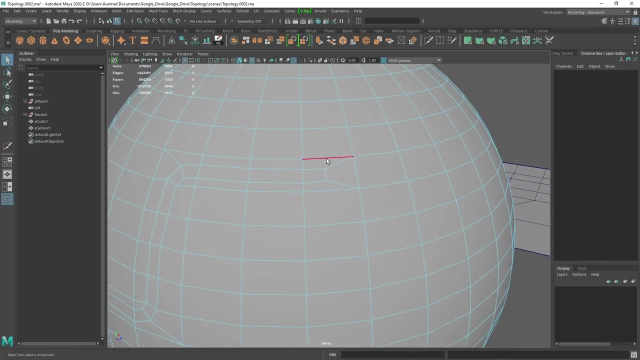 Now, of course, we see how this ends up. you can easily fix that by going into multi-cut and using that technique that I showed on tip one. So now, if I go ahead and just kind of cut this across like so, and then I cut it, cut it and meet it at these corners here, there you go, You get. 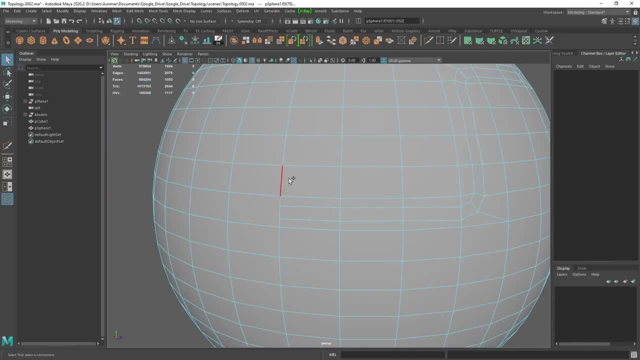 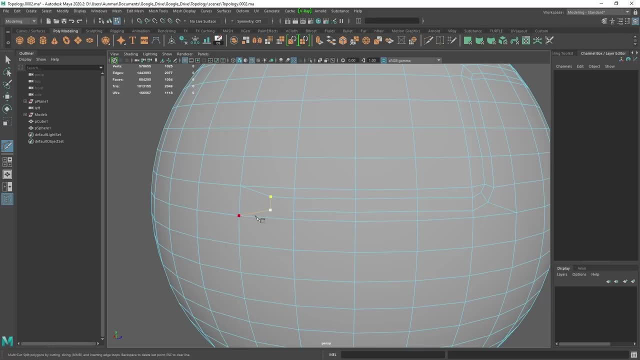 nice quads here, which is exactly what we want, and then you can terminate it here like so, and this is just one way to do it, right. So here's just another way of cutting it, which is just a few more clicks, but it's all the same at the end of the day, Okay. and then we get this nice face. 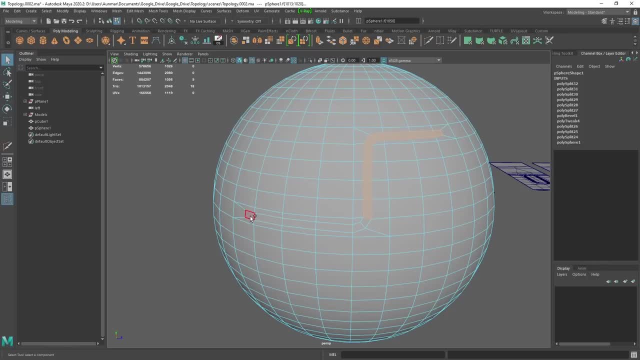 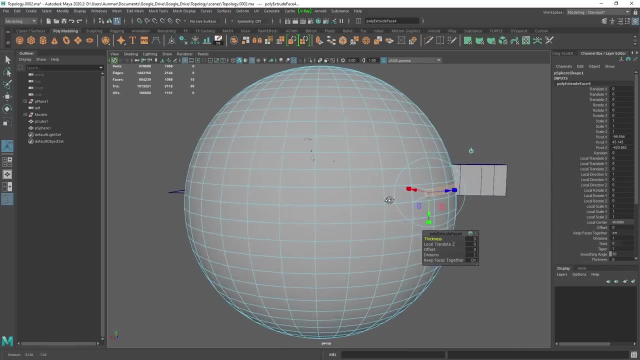 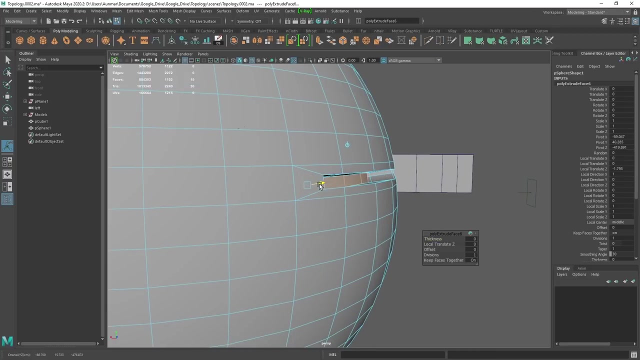 loop here that's running all the way across our model, So I can click, click here and grab these and then I can do a control e for extrude and move these in and g again. just give myself a little bit of a holding line and I'm just showing an example of 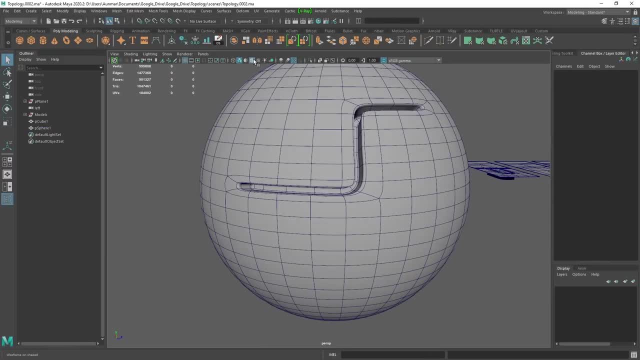 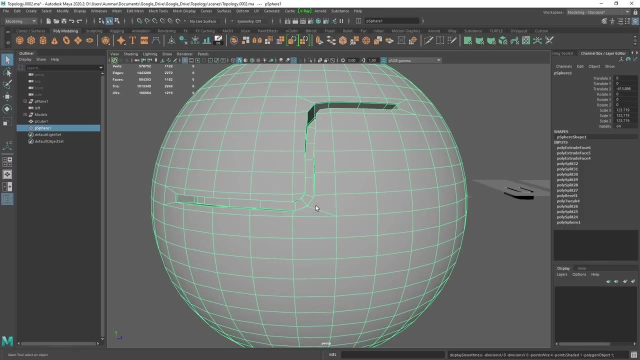 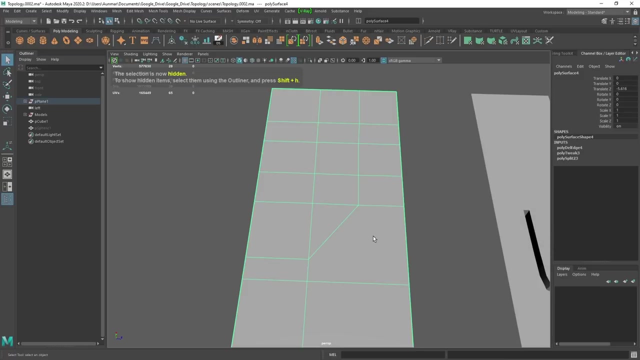 how to just kind of cut in on an organic surface. and there you go. So now you can see that cut in pretty well and I'm able to add in these nice corners and clean those up and still maintain quads by splitting that quad, excuse me, that triangle and that end gun. All right, the next. 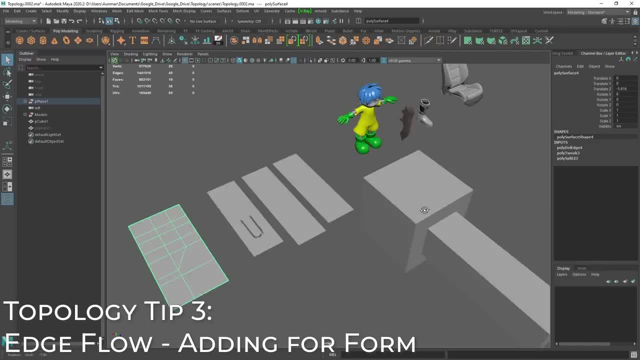 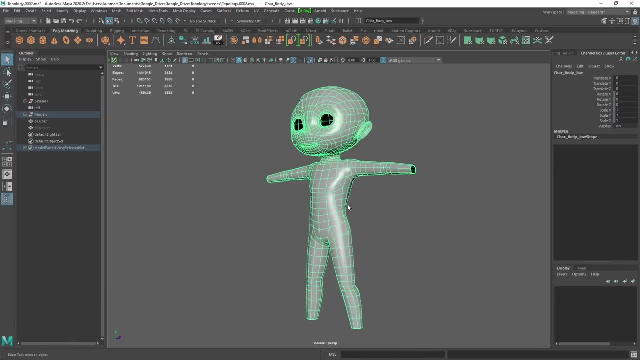 tip I'm going to recommend is edge flow and keeping an even distribution of edges. If we take a look at the model here as an example, you can see that this character model that I've created has a nice clean, even distribution of edges and that everything. 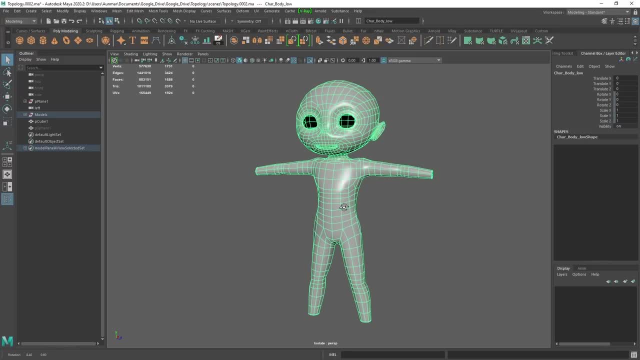 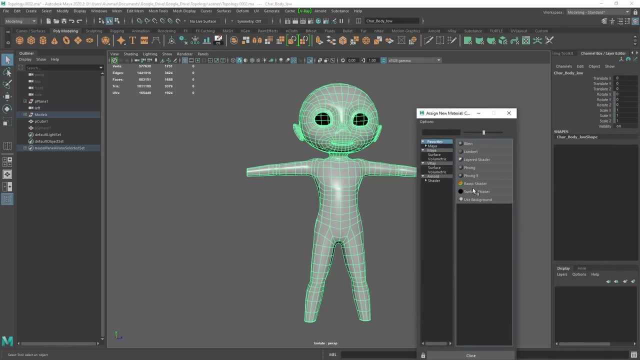 every edge that's in here is helping the form. Okay, and what do I mean by that? if I actually go and select this mesh and apply or hold right click- just simple right click- don't hold, shift or anything- and assign a new material, I'm going to assign what's called a surface shader. Now I like 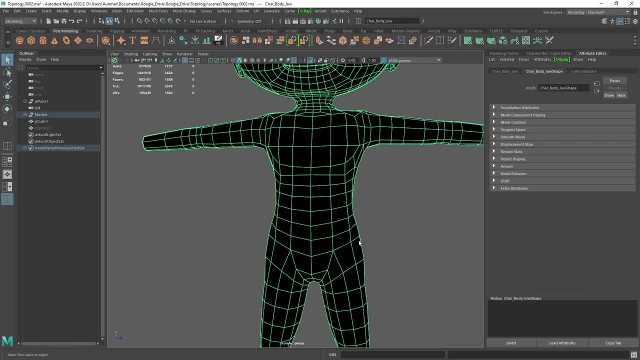 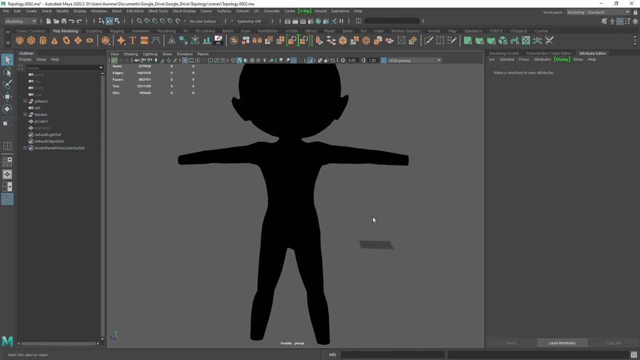 to keep this kind of in the center, because it just lets me know where my edges are being most impactful and if I have any dead edges, and it just allows you to look at the silhouette of the model and focus on the form. If you notice, you have what's called dead edges. so, for example, if I 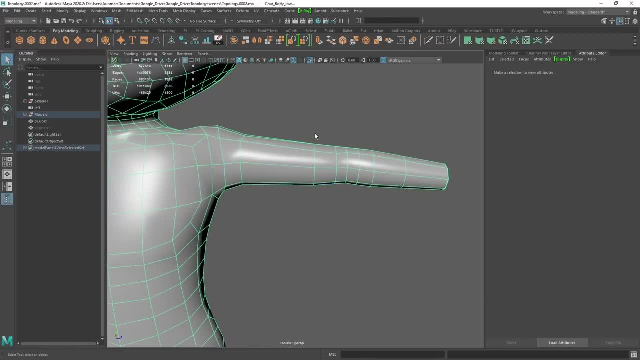 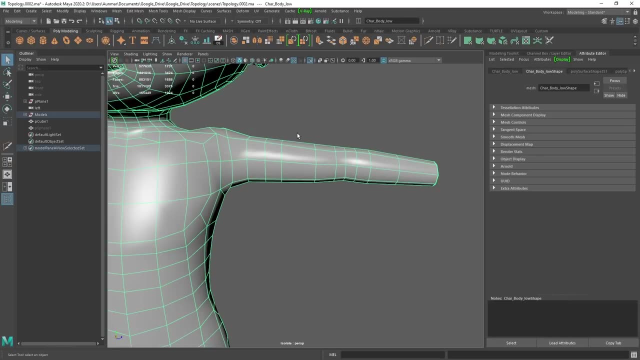 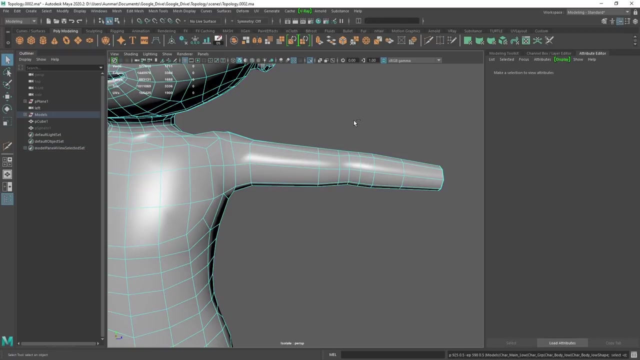 take this and delete these. you can see, now I just have straight edges here and then if I multi-cut and maybe add in a couple of cuts, now look at the difference, right, look at the difference. this, which is super flat, which is again kind of those dead edges that I was talking about. 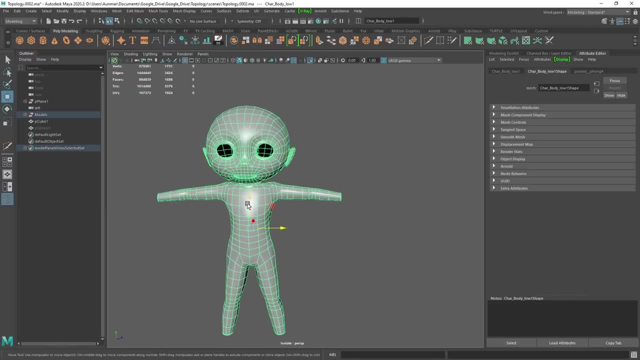 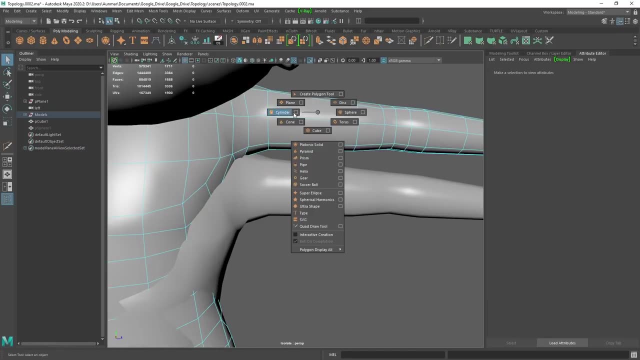 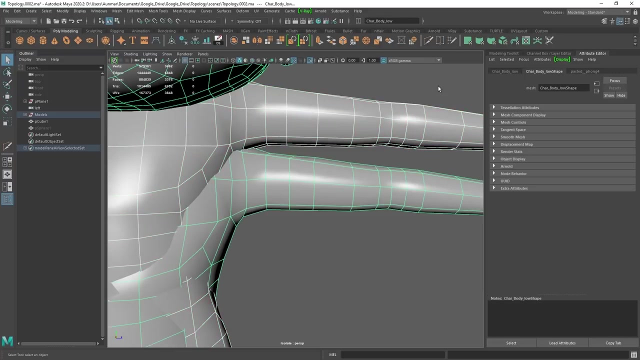 right. So if we go ahead and maybe duplicate this and move it this up like so, And I'll remove these edges, And you have to be careful, right, Because sometimes you're just going in and cutting and adding things but not adding to the form, That's where you run into issues like this, All right. 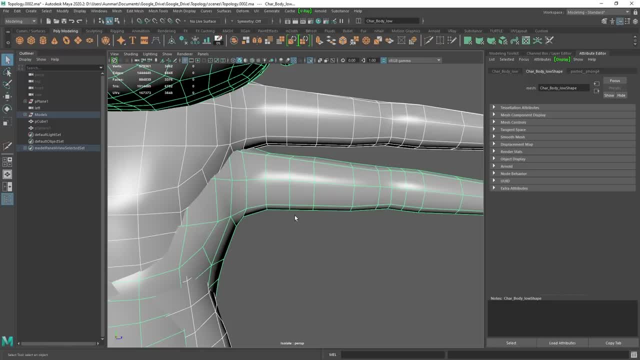 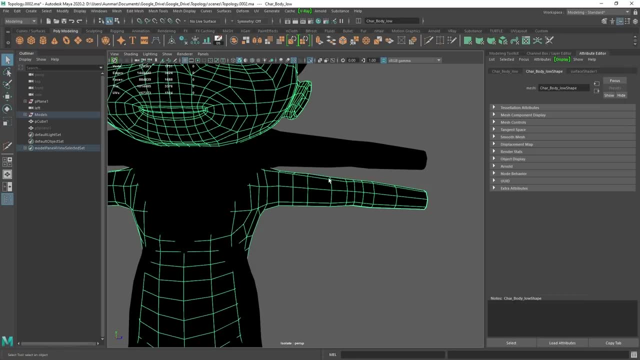 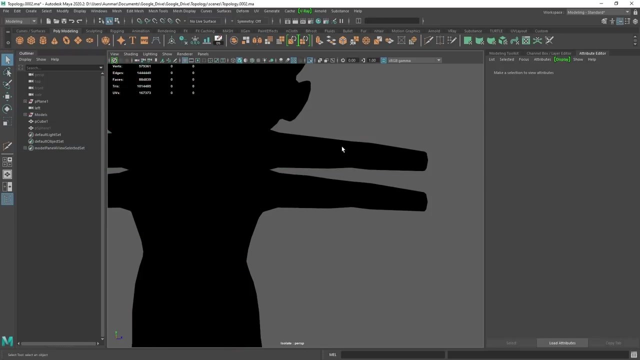 And then I can do assign a new material and assign the surface shader right, And you can see that here I'm getting more depth, more form out of my edges. here versus here, which is a complete straight line. It's very subtle, But these are the things that I'm looking for as 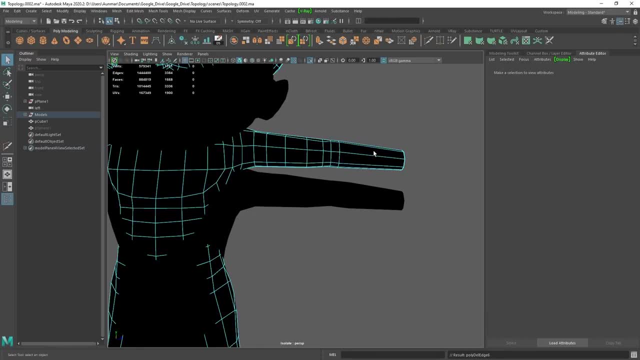 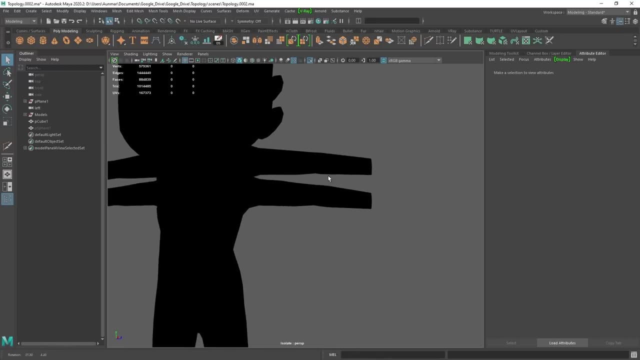 I'm going through and working on my models, right, And so you can see if I do the same thing here. our arms now are super straight, right, Very tubular, All right. So you definitely want to keep that in mind, and even distribution of edges and adding. 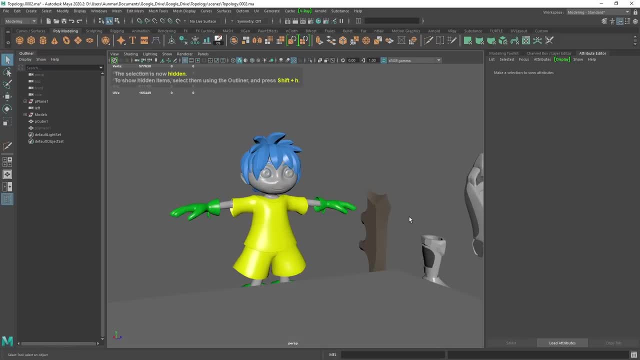 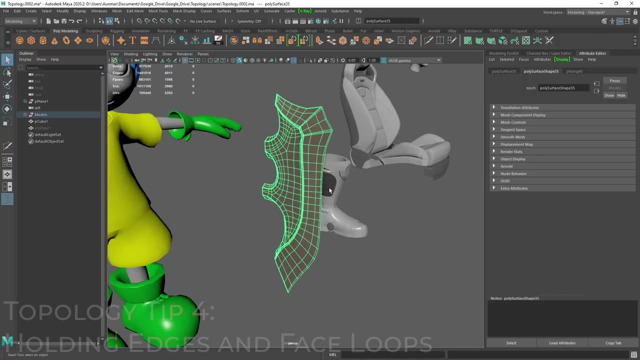 edges as you go, Right. So I can take a look now and kind of see you know this here with this, with this tip, right. So now I have the next tip, which is going to be holding edges and face loops. 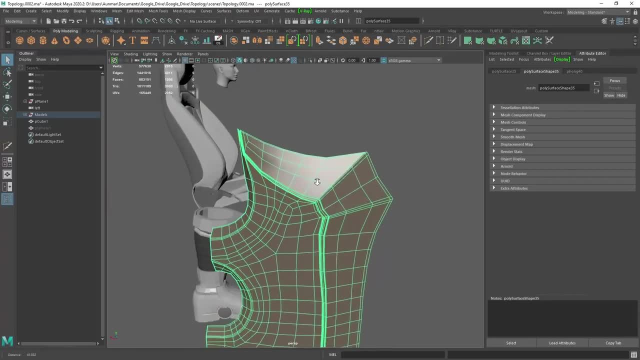 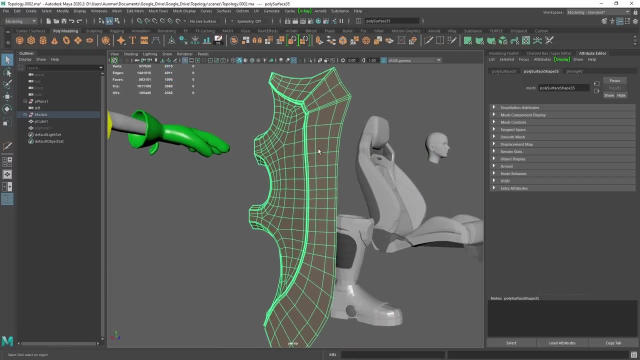 So edge flow here, you can see, is really important And especially when it comes to holding the form, you can see, I have this fairly organic looking axe shape And I have, just like the last tip, a good, you know even distribution. So that's being applied. 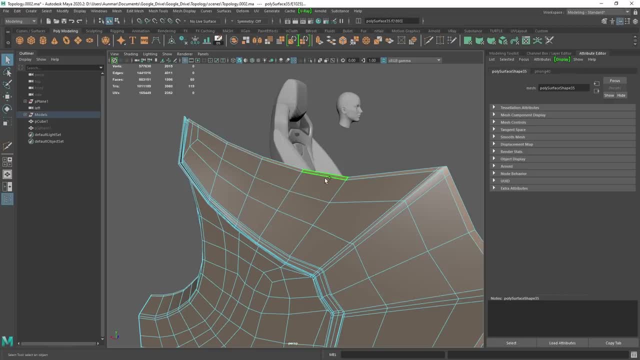 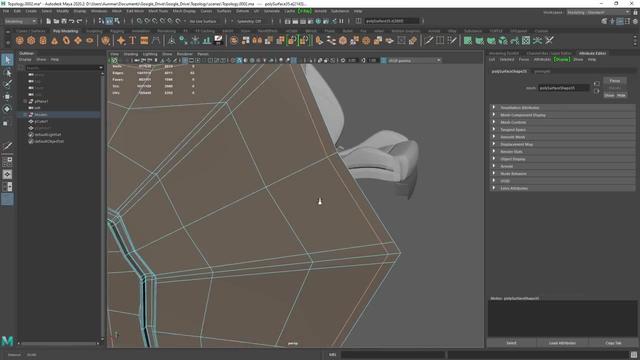 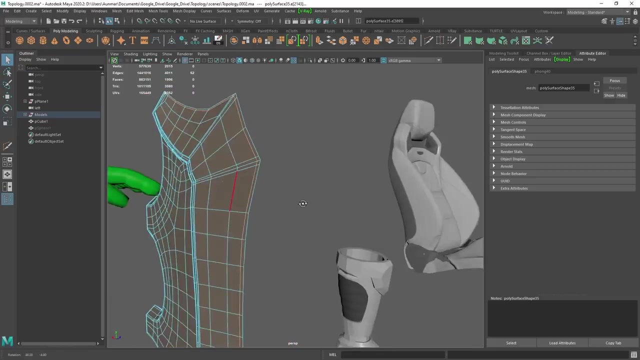 here as well, And then I'm having these holding lines that's being applied to my models. A lot of times I'll see people- you know, students and whatnot- create models and they won't add in these edges to hold form. So you always want to make sure to add in those good holding lines. 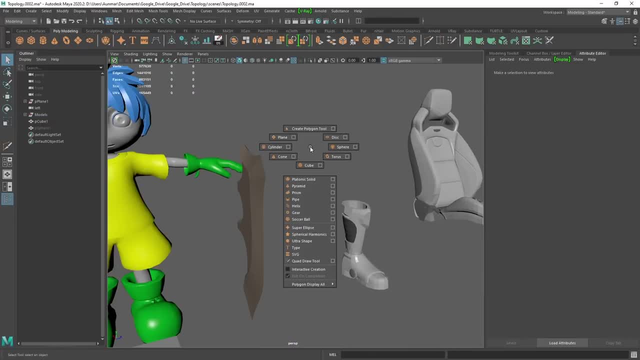 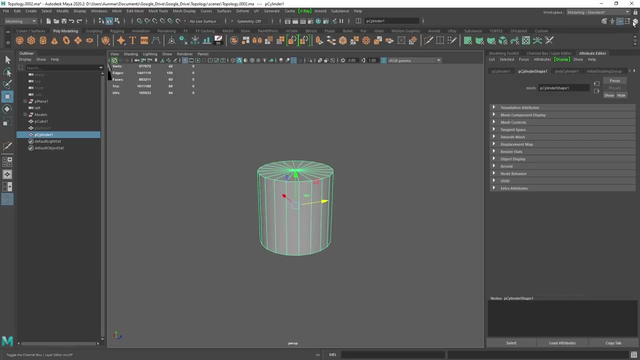 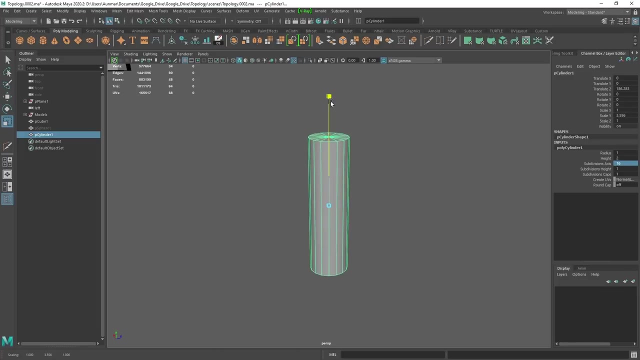 on your models In the simplest form. I can go ahead and create a cylinder here and bring this over, And if we take a look at this and I can give this, you know, maybe 32,, maybe even 16, right, so you can see it kind of working more impactfully. So if I have 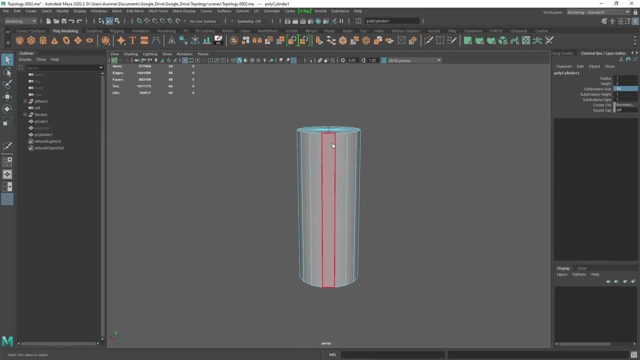 something like this and just right off the bat, if I go ahead and hit three for smooth preview, I've lost that form right. So that's where your edge flow and holding lines are going to come into play. So if I go now into here, you know, and grab my multi cut tool, I can add a multi cut here at the 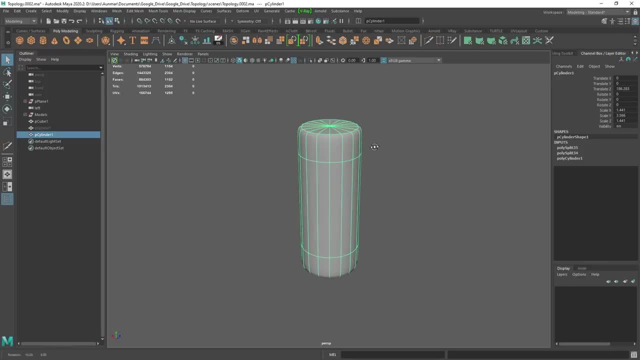 top and then here at the bottom, but then watch what happens. It's starting to get better, right, But I still need a little bit more. So if I apply a font here, you can see how kind of soft that's looking right. So imagine if this was an arm or a piece on a hard surface model. 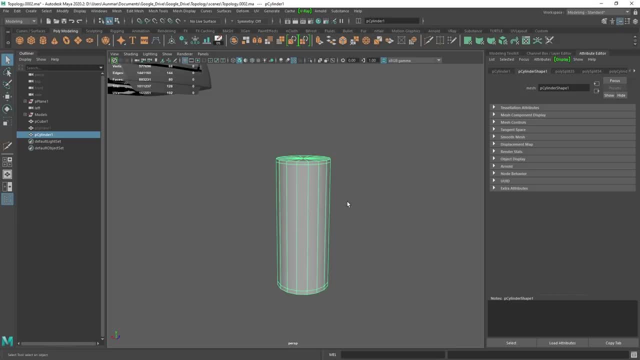 we need more geometry. I always tell students: don't rely on smooth preview for your form Meaning. you need to add in geometry and the mesh smooth that happens at the end. this really should just be kind of like if you were applying this, this soften edge, at the end. That's how you want. 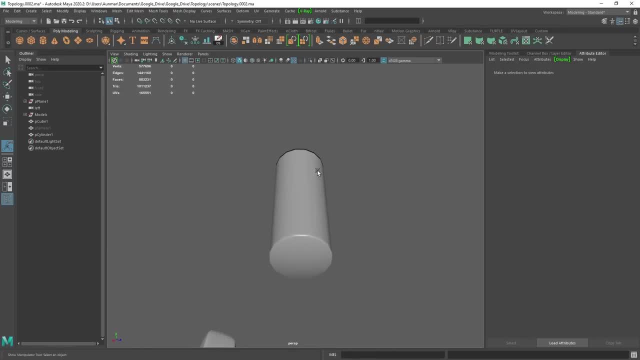 to look at it. you don't want to rely on it for your form. So you can see we still need a little bit more here for the subdivision. So what I'll do now is go into face mode, select these faces here at the top and the bottom. 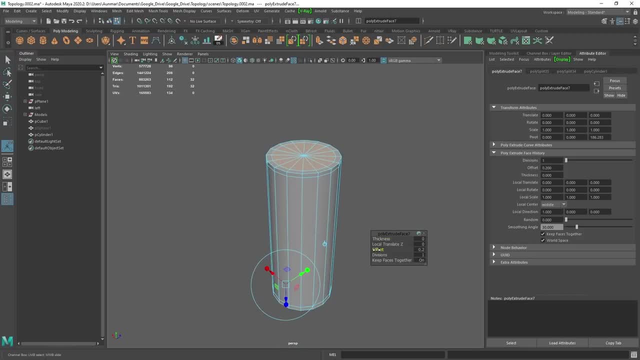 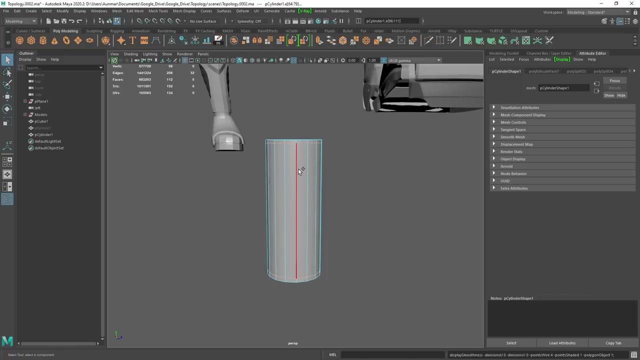 Then I'll extrude these faces and then I'll do an offset. So now I got these, So this is getting better. so I'm holding the form from the top and the bottom, But then I also need now look what happened to these edges. they're coming closer together, So I'm going to need even more edges. 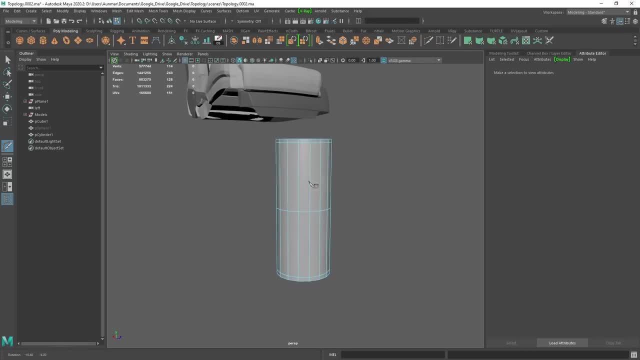 here in the middle for this to better subdivide. So for now, if I go ahead and just control middle click about two to three times, so I'll do it three times Now. look at this. you can see how much better its playing. It's getting even smoother Now. I'm doing the same thing right here and 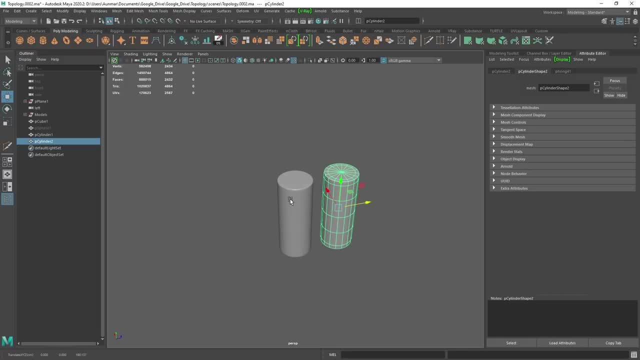 this looks and if i go ahead and duplicate and move this, this is the sub d model, or the subdivided one, the smooth preview. this one now is going to be the softened edge right. so you can see that now they're much similar here in overall form, versus having something where we 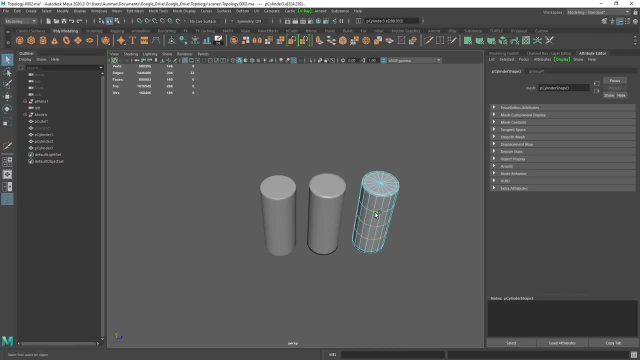 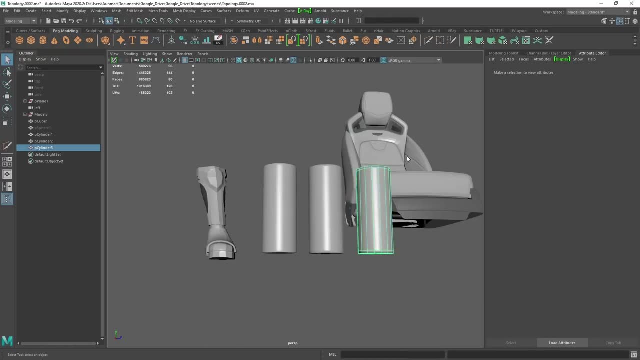 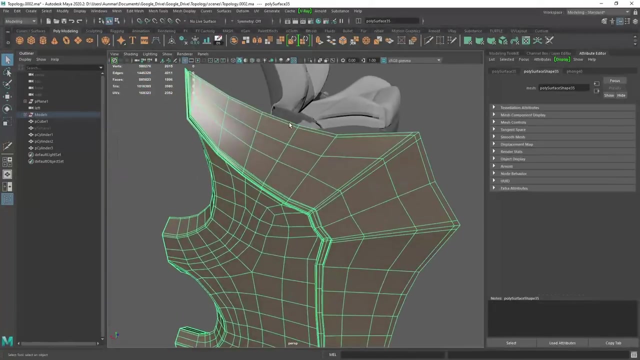 originally started, which was, you know, not having these holding lines and the holding edges. now this is, again in its simplest form, how i would apply this to a cylinder right, so the same can be applied to more complex models here. so definitely looking for these face loops here for holding the 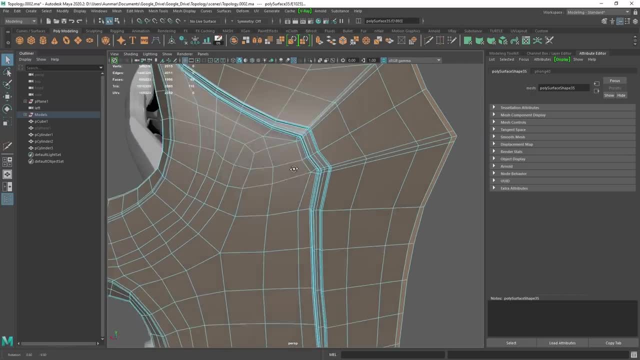 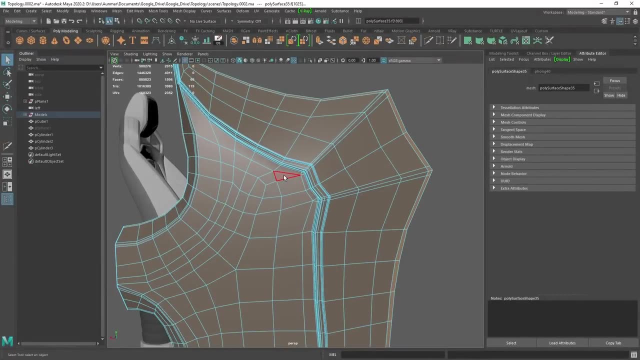 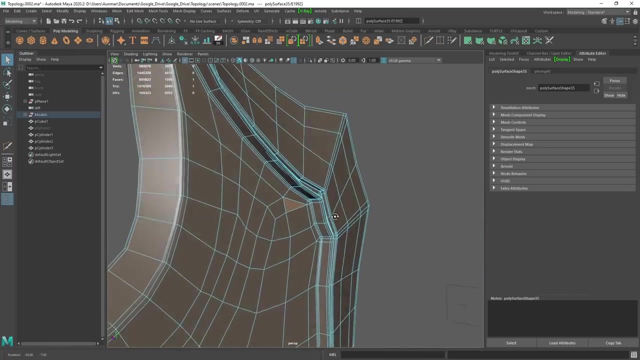 form. we have our holding lines here and then you'll see the kites and everything coming in. now i did want to add in: i left this triangle here so you can get an understanding of sometimes having triangles are completely away okay, especially with hard surface and flat objects. so don't worry and don't try to kill yourself to. 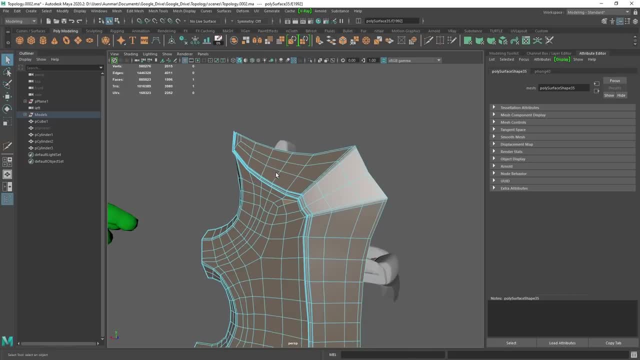 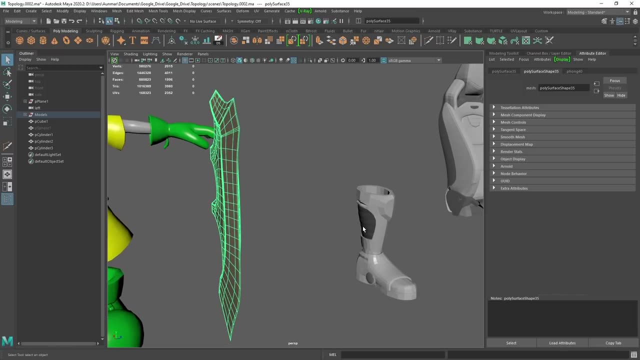 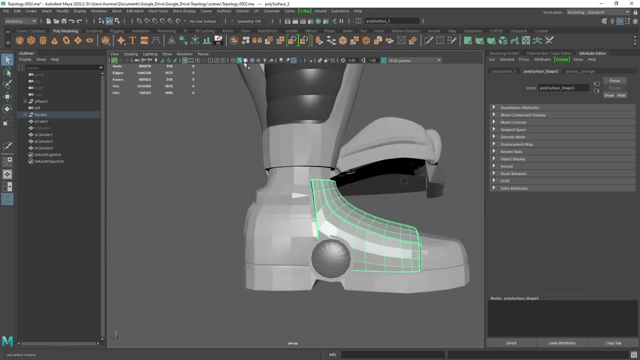 try to get all even quads. sometimes a simple triangle will will keep things just cleaner even without having to cut in and add more geometry. all right, and so you can see another example here where, if i turn on edge faces here, you can see that i'm using these kite quads all over the model. 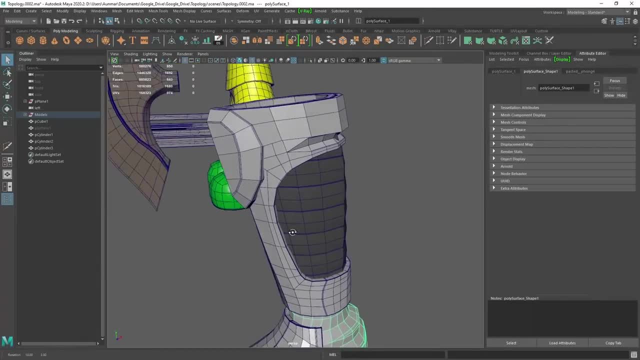 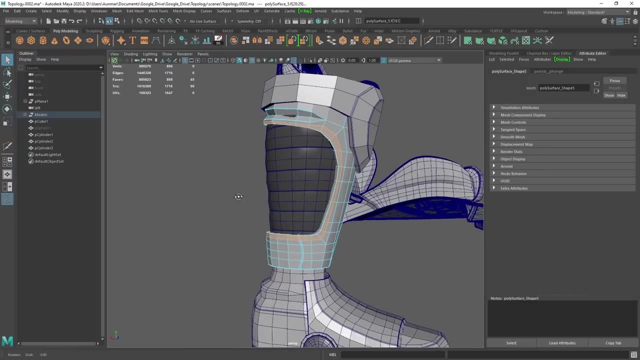 here. this is kind of on a boot, on a character that i modeled not too long ago, and then we can see that we have these face loops here, these holding lines. you know, that's just holding the overall form right, because without that that's not going to hold the form. 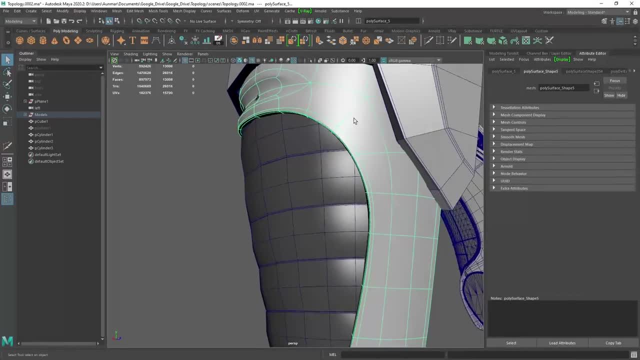 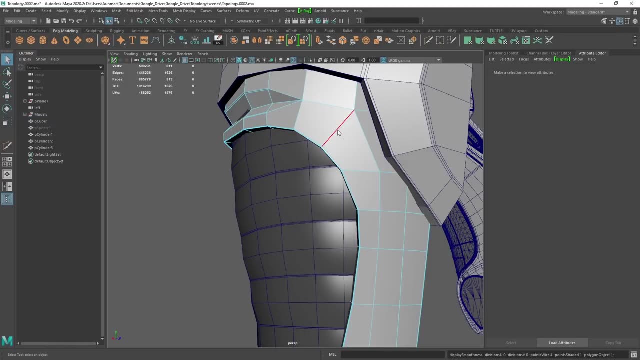 as well. right, these are the subtle differences between you know, having and not having these things. so you can see how the difference in the spread here when it comes to sub d modeling and topology- and if i re-add that you can see now it really keeps this edge tight. 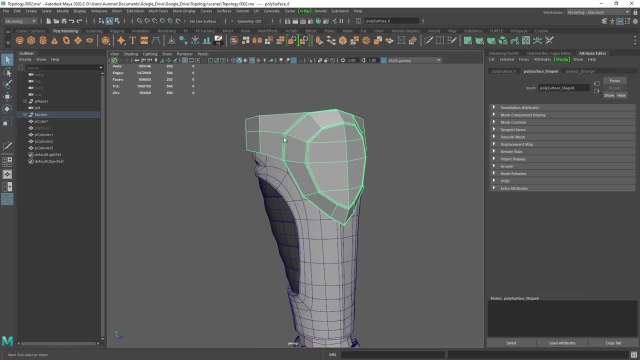 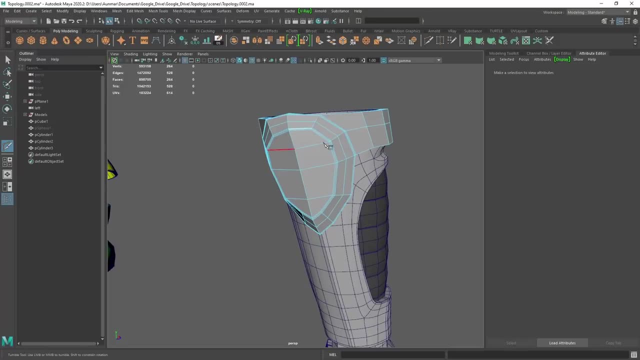 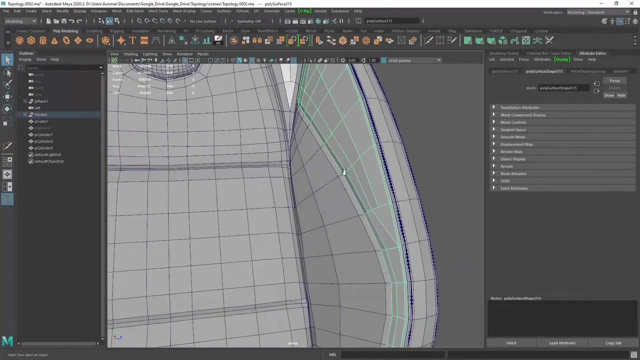 tighter here, All right, And I was actually in the middle of this one, So this one needs a little bit more holding lines. but I left it like this So you can kind of see exactly what I'm talking about here, All right, And then you can see more examples of how I use kite quads, especially when 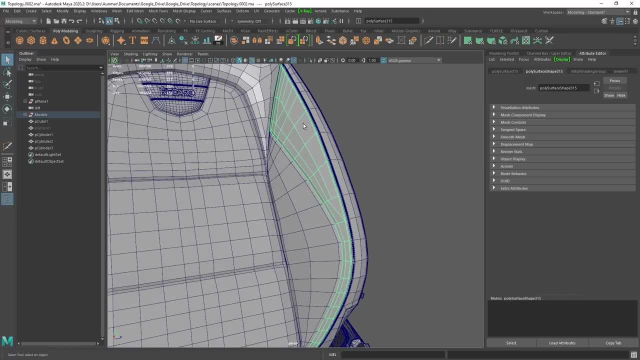 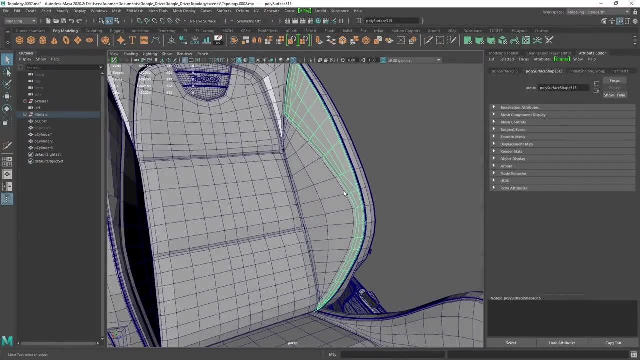 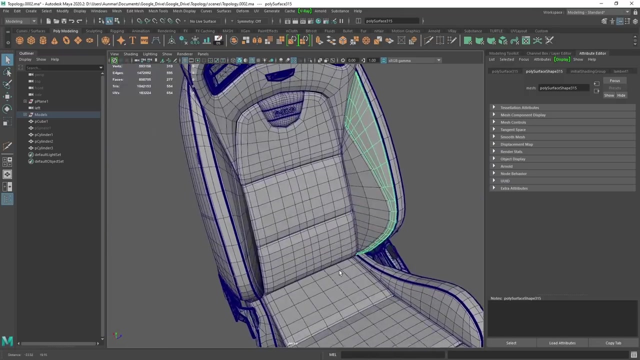 you're, you're working with larger faces that have to come down to really, really thin faces here. So this is a Recaro seat, a racing seat that I modeled for a vehicle, And you can see exactly that technique and that edge flow being put into practice here. All right, So these are the four. 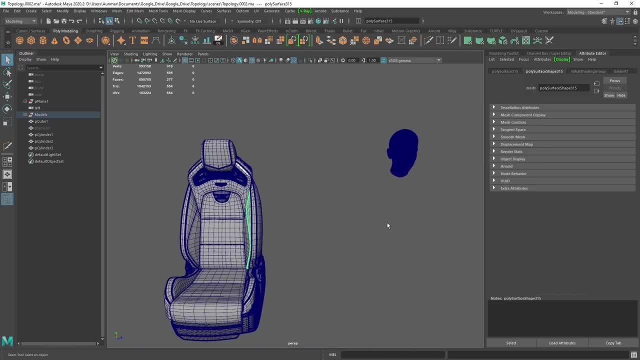 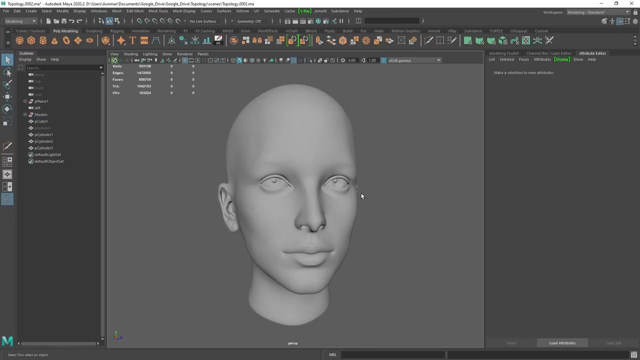 and the last one, the fifth technique is is going to help you improve topology almost immediately, And it's going to be practice. you know, practice topology. But what I mean by that is, you know, focus on just re-topologizing, All right. So what I mean is: take a look at. 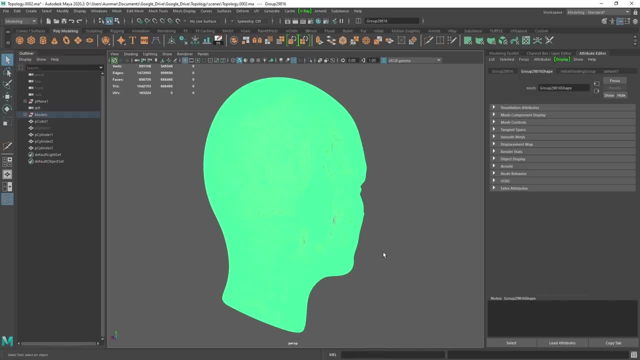 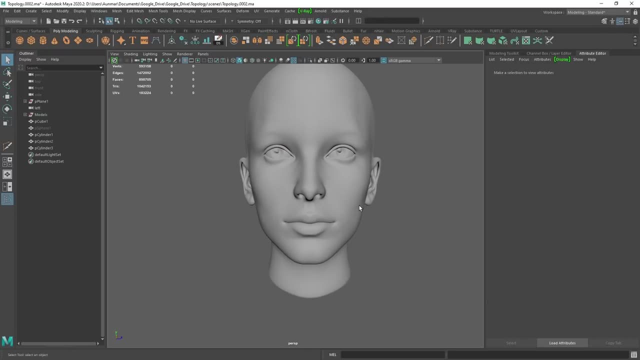 I just pulled this model, this head sculpt, from ZBrush and I just decimated it down and I brought it into Maya. Find some models that you've done in the past, Okay, And if, if you're struggling learning topology and edge flow work and use the tool called Quadra. So what I'm going to do now. 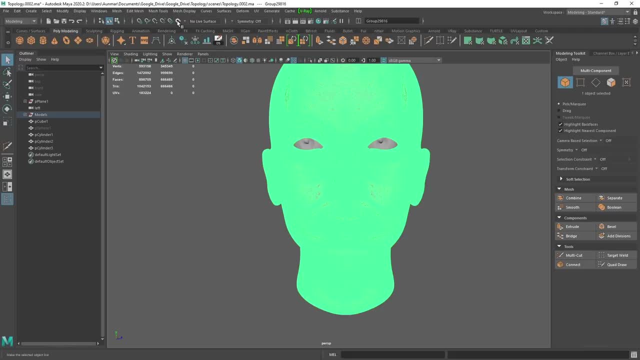 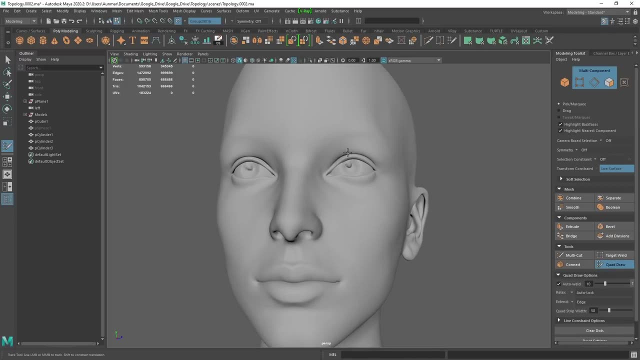 is: select this model, go ahead and turn it into a live surface, And then I'm going to use Quadra. Now, what Quadra is going to do is allow me to start plotting points, So I can left click here four times, shift click and boom, I've created a quad. 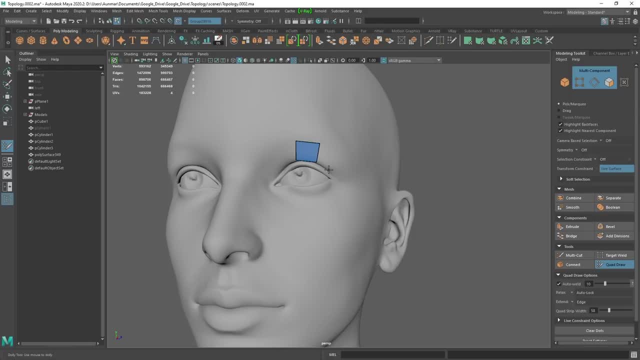 So you're drawing quads on the surface, Then I can just continue to do this and then add two. And in order to get the face, you, you plot the points. hold shift and left click. Then you can also hold control, left click to add, or 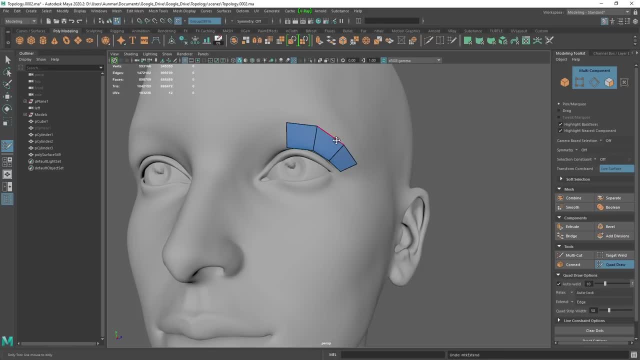 hold tab to pull out some edges. Now you can use tab and middle mouse to pull out edge loops, or if you have an edge in here and want to get rid of it, then you can hold control, shift and delete. Those are the main ones that I use, but take a look here in the modeling toolkit and you 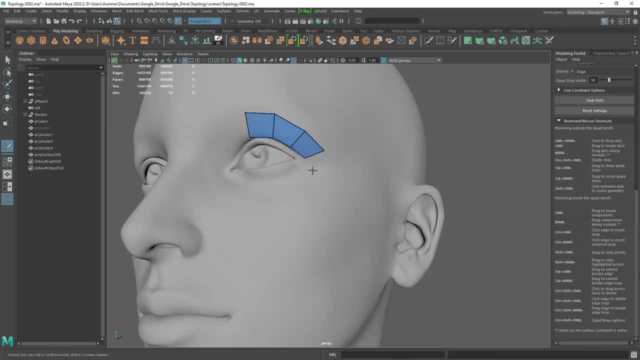 can see the keyboard mouse shortcuts, and there's a ton of them here. So now that I have a model, that I don't have to worry about form, I can just practice topology, And then not only practicing but also doing some modeling. So I can just do this. So I can just do this. So I can just do this. 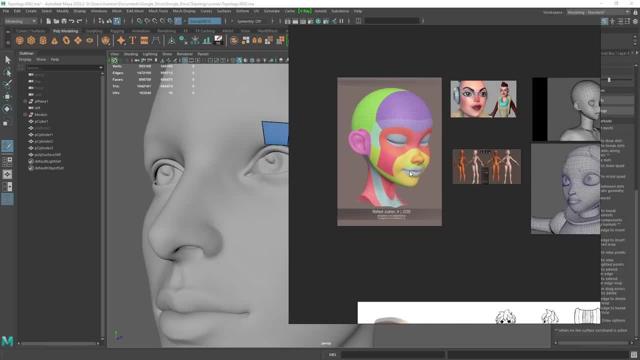 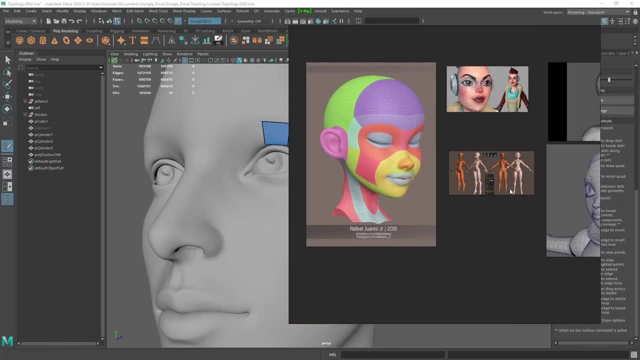 But if you take a look, you know I've I've covered this in the the hammer when modeling series that I did. but you want to make sure to reference topology, good edge flow. Here's some samples that I just pulled off um just from the internet. when searching for good topology, 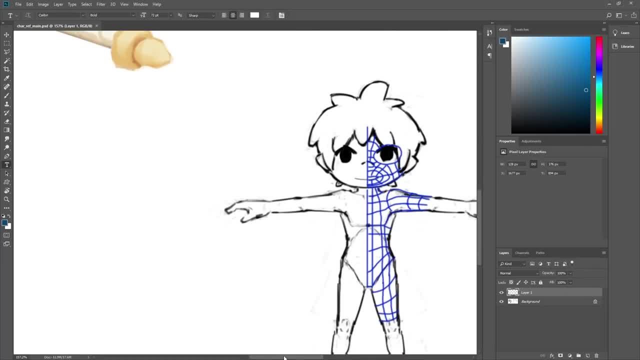 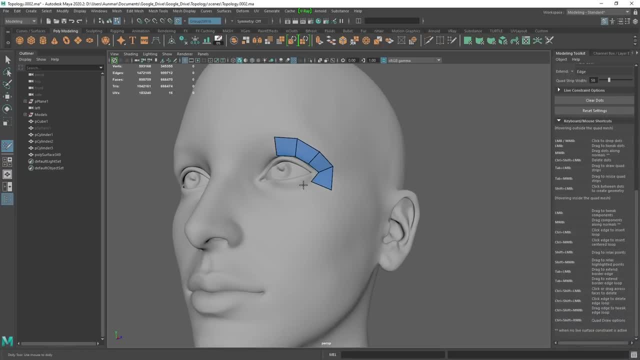 And then I'd also just do some sketching right, Sketch down the topology, just kind of plan your topology. Then you can get back into Maya and just start working on you know, having the the you know ability just to focus solely on topology. And when I started doing a lot of 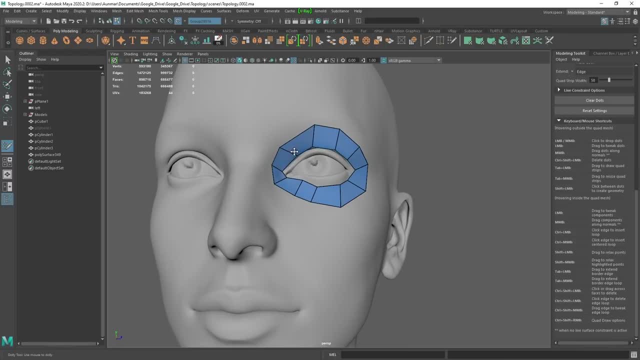 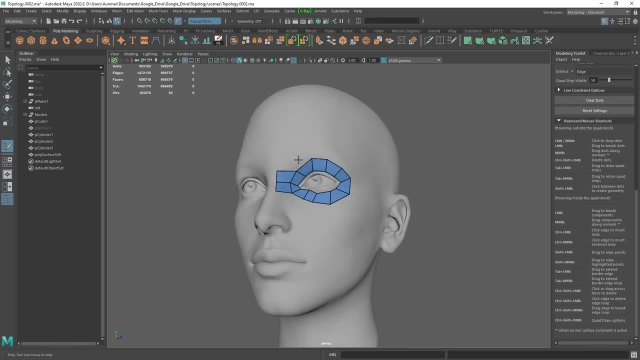 retopo work. that was when my topology game just immediately, immediately improved, Right. So, and it's just one of those things I'm not saying you know, just you know, cause that's the whole workflow of being able to sculpt and then retopo, um or create. you know, very high. 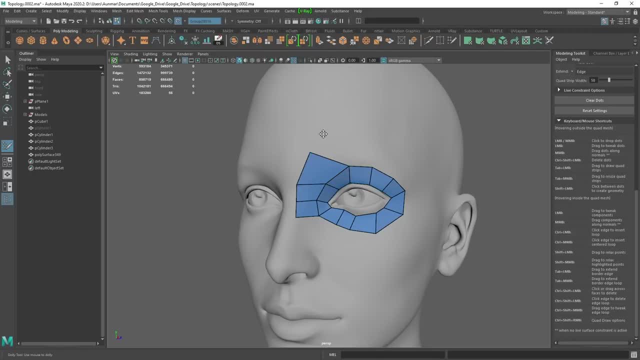 high detailed models and then retopo later And uh, so you, you, you have these types of uh workflows, right, And so you know, you you're starting to work on the eye loop and then now you're working on the face loop, um, or the mouth loop here, Um, and you're just kind of going. 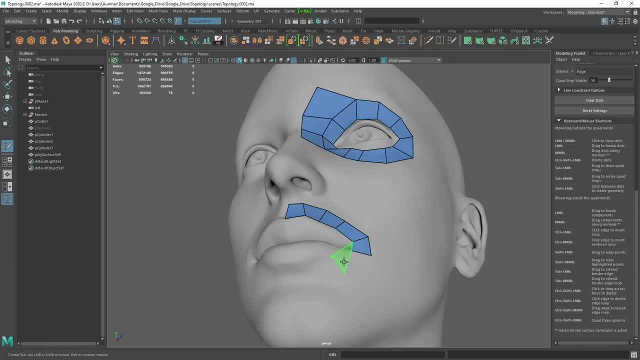 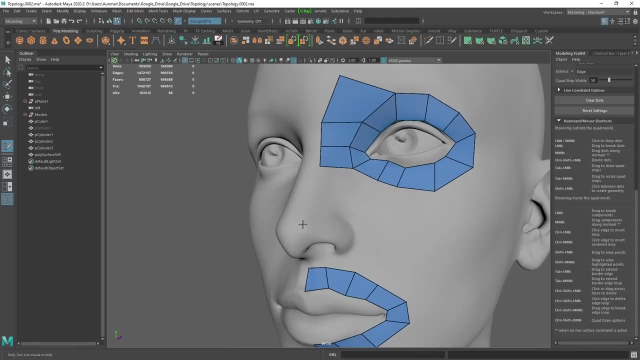 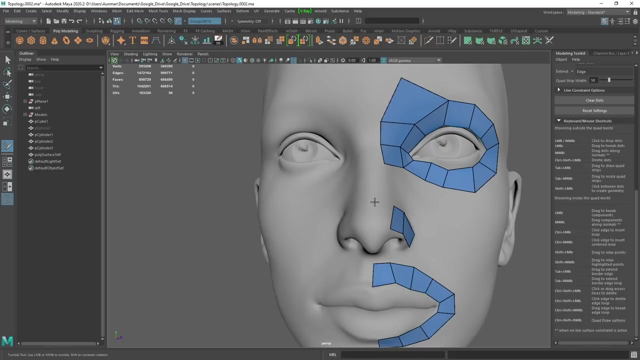 around working on, uh, the model right. So this will allow you to just again focus solely on topology and edge flow and allow you to to get a lot of um ground covered there. It's kind of that focused, focused practice. 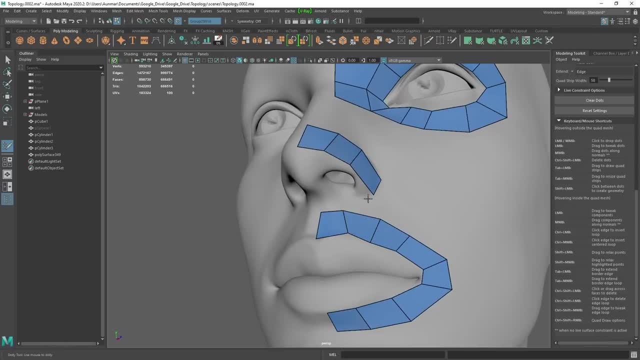 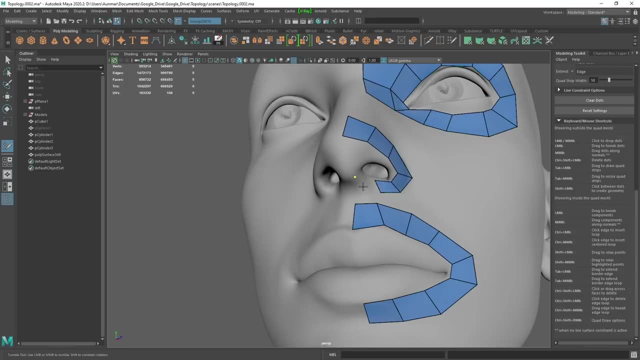 And when you get back to the regular modeling with your- you know the regular modeling where you have to do everything, then that's where it's going to be, you know, helpful, where you're starting to combine all those techniques Once you start becoming really, really proficient. 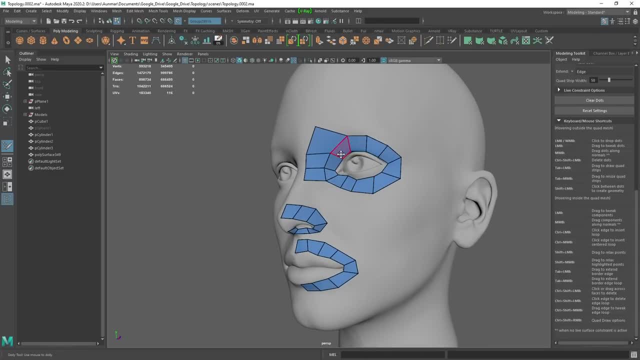 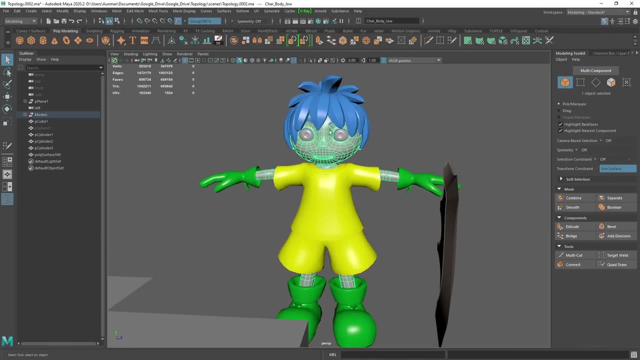 at topology, right? So you can see I'm just kind of going and looping. but you know, you don't have to pull in sculpts, You can simply take old models that you've done. So here I have this. 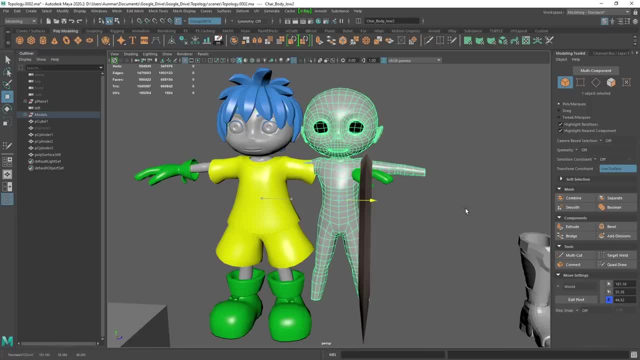 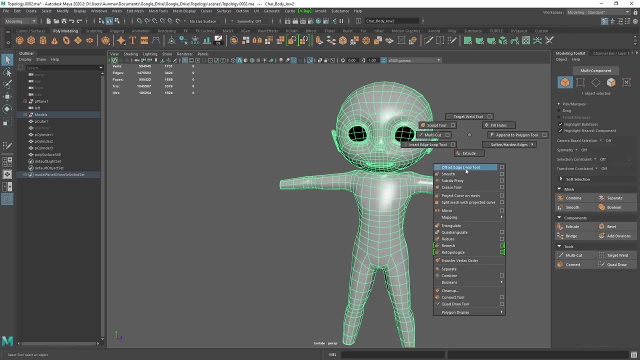 character model that I did. Uh, so I'll move him over, duplicate them and then, uh, I'll get out of make live mode And what I can do here is subdivide him a couple of times, like so. and you know this is. you know I can. 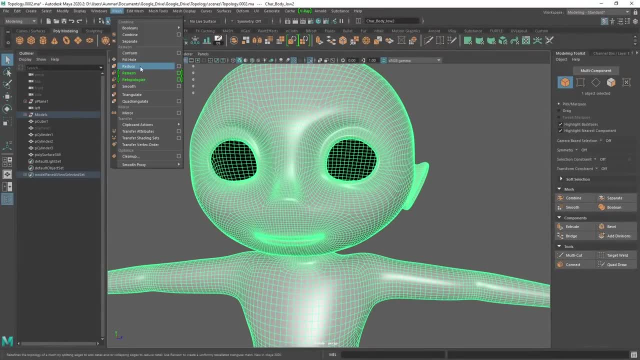 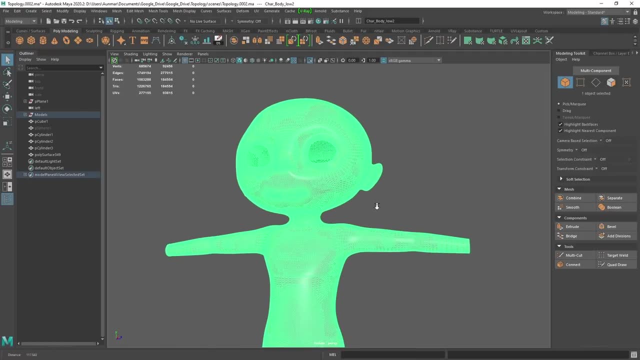 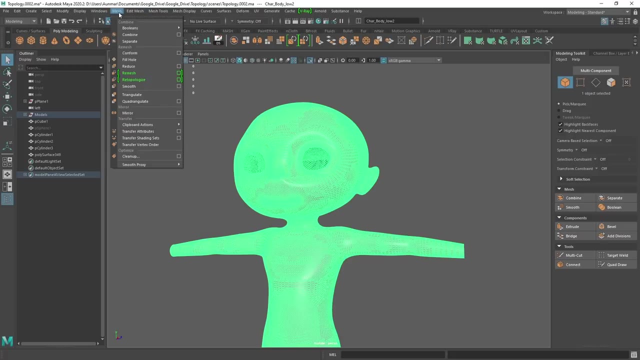 work with this, or I can go in here and do a remesh like this, And so now we just get like this messy topology version, re topologized version, uh that we can work with. Or, you know, you could even use the uh optimize too, which is going to uh really reduce the. 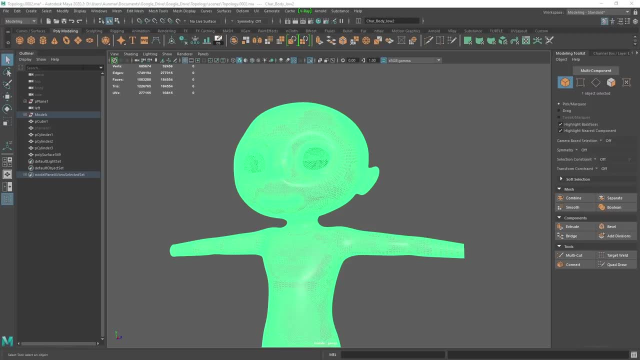 the mesh here And you want to get that by going to mesh reduce and then you can say like, if you know, 50% or whatever, and then apply that And that's really going to change the topology. And the whole purpose of just doing this is so you have a completely remeshed and re-triangulated 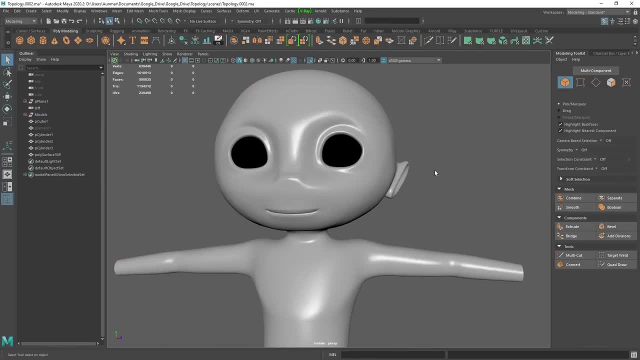 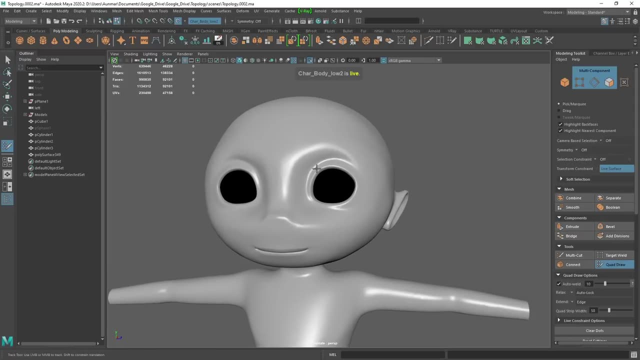 version uh of your model. So that way, you know, you're not, like you know, trying to, you know, to carry over the bad topology that you had previously. So then, yeah, I can go ahead and make this guy live and I can quad draw and I can just start, you know, start working um with him. 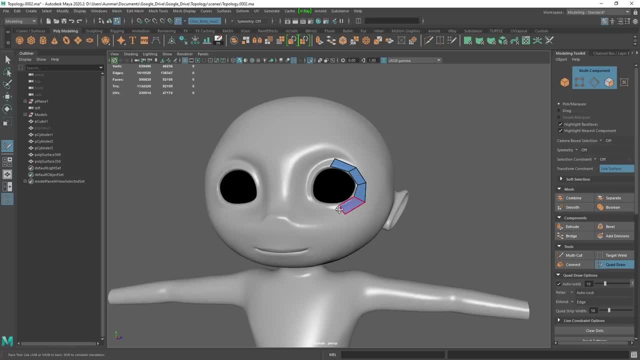 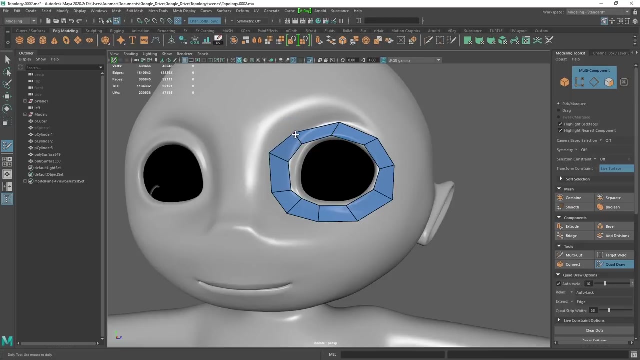 uh here, All right. So definitely using this to practice your topology. uh, use models that you've created before, use models from your friends or models you find from online, And it's just going to help uh things overall All right. So that about covers it. Those. 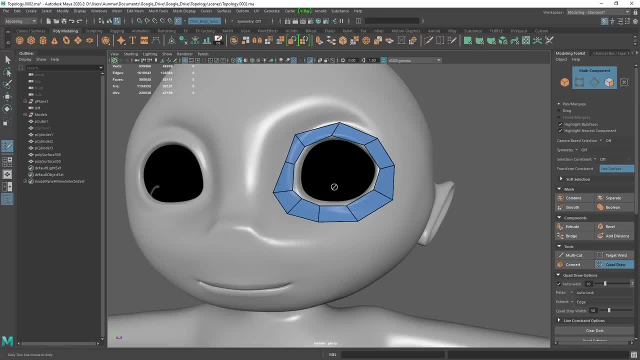 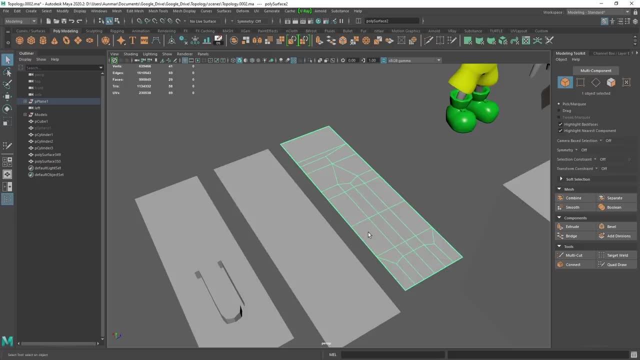 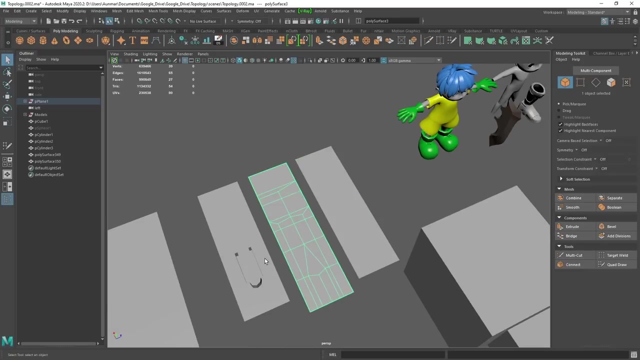 are the five tips. So, to recap the five different tips, the first one is, uh, localizing topology. So I go over here, that's having the ability to take one face and convert it into, you know, three, four, five, six faces and going back down. uh, all the same, right, So we're doing exactly.